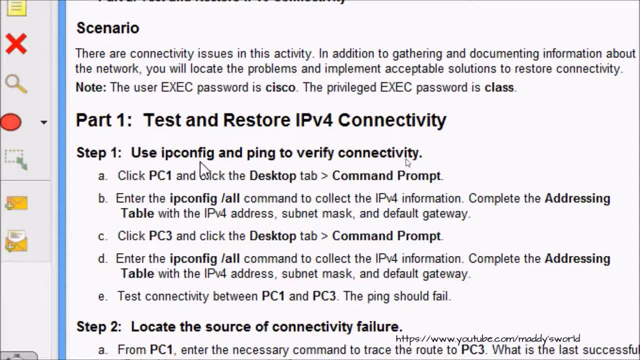 connectivity. In that step one I use ipconfig and ping to verify connectivity. Click pc1 and to click the desktop tab command prompt. enter the ipconfig space. slash all command to collect the ipv4 information. right, we have to get the information from pc1. complete the addressing. 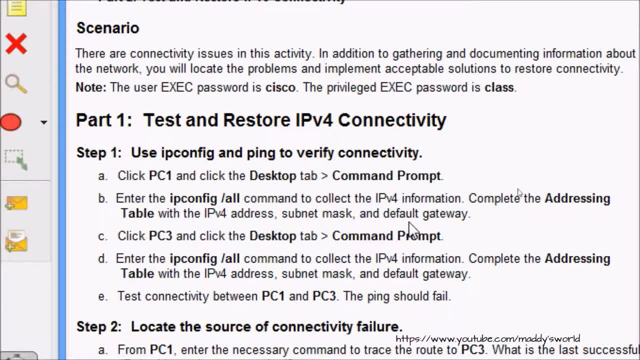 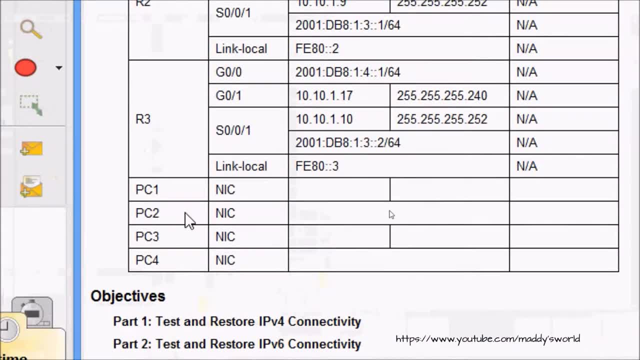 table with the ipv4 address. submit to mask and default gateway. yes, if you observe this addressing table here, we can see. we have to complete all these informations. you have to collect information from pc1, pc2, pc3 and pc4 and we have to update this table right. 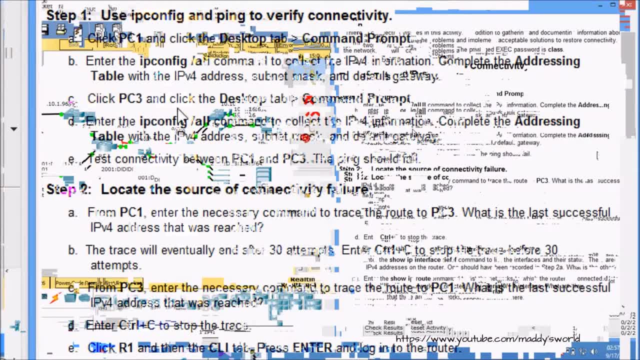 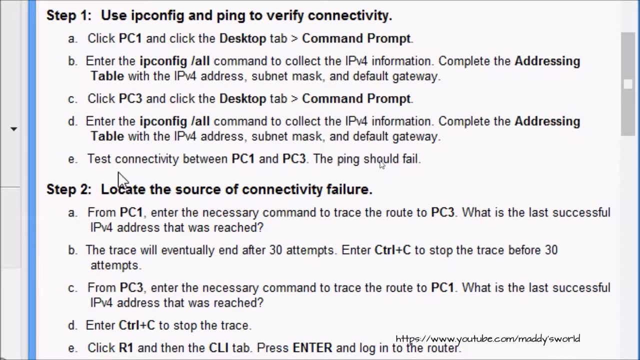 also we have to collect the information. click pc3 and to click the desktop tab command prompt. enter the ipconfig slash all command to collect the ipv4 information, complete the addressing table with the ipv4 address, submit to mask and default gateway. then finally, we have to test connectivity between pc1 and pc3. the ping should fail, right. we? 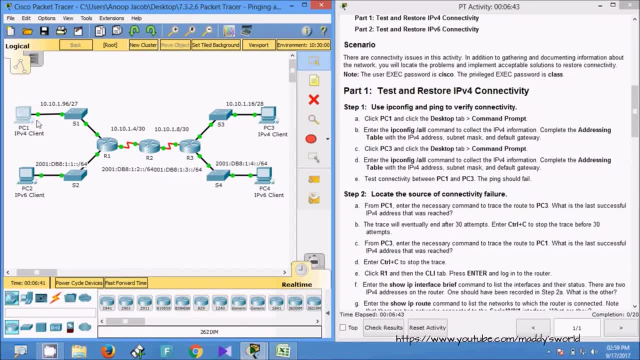 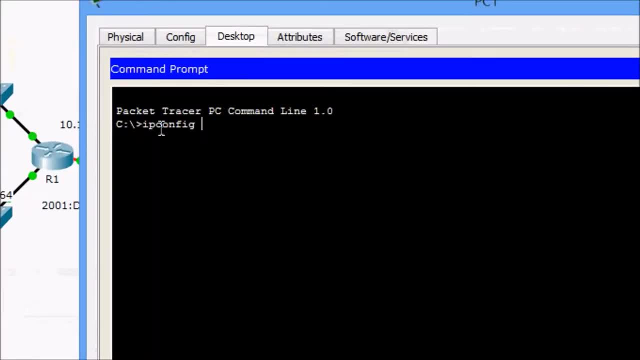 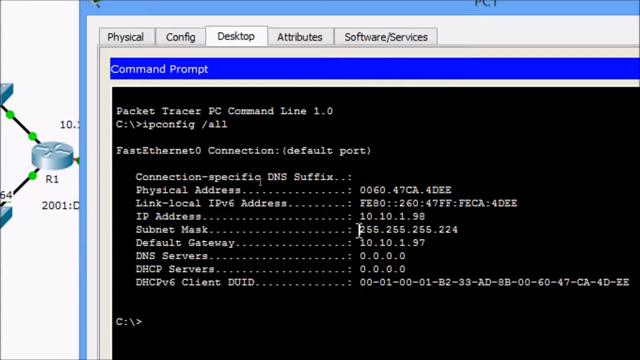 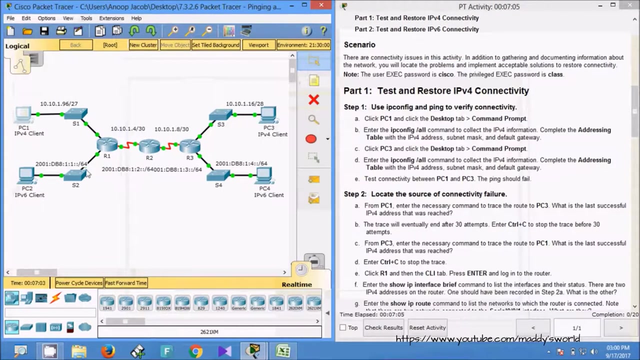 will do this now. here is our pc1. we'll go to desktop command prompt. here we are going to give ipconfig all and here we can see the details. ip address: here we can see the submit mask and here is the default gateway right. also we will verify on pc3. 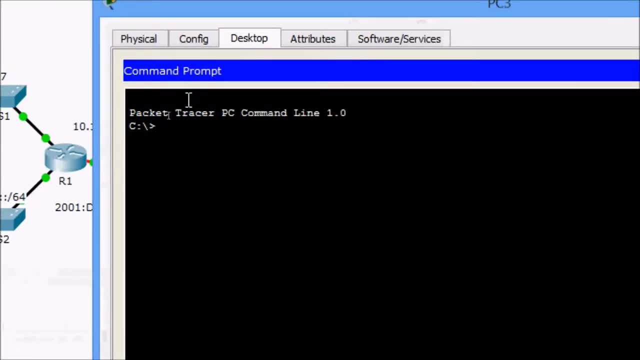 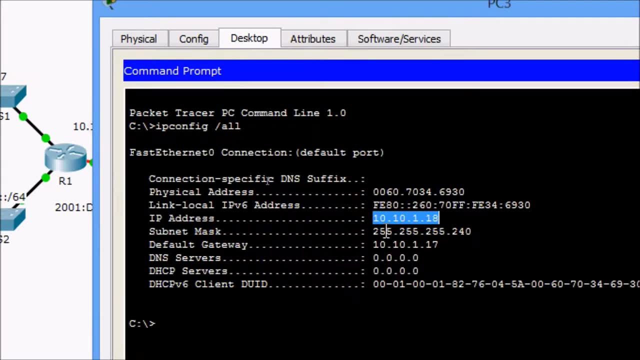 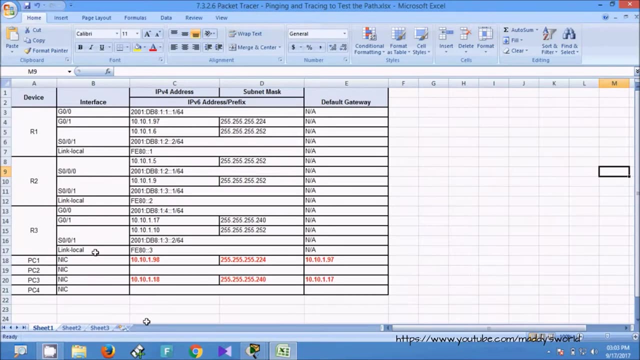 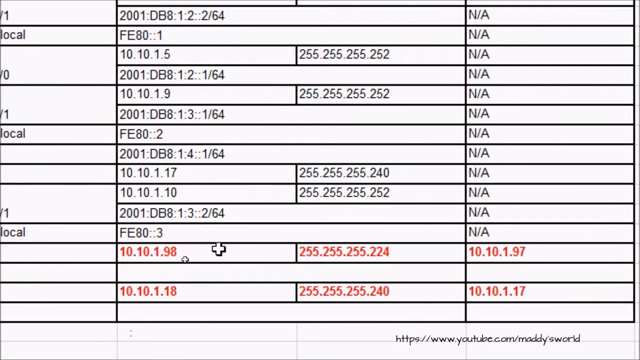 desktop command prompt. here we are going to give ipconfig space all here we can see the address, ip address submit to mask. also we can see the default gateway. right here we can see our addressing table and we updated the details of a pc1 and pc3. here we can see the ip address submit to mask and the default gateway. 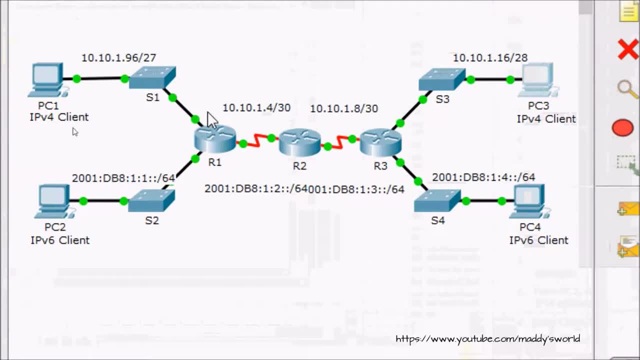 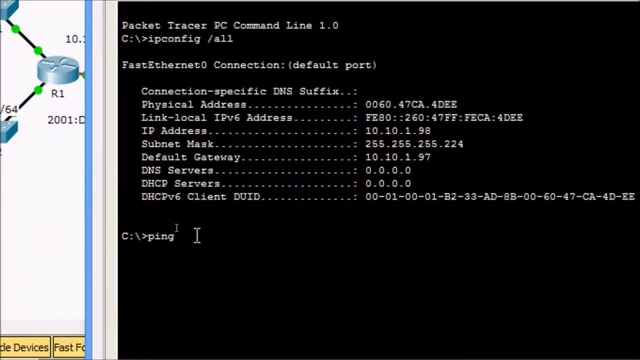 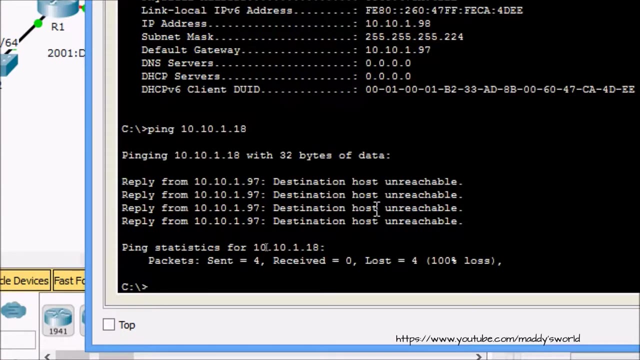 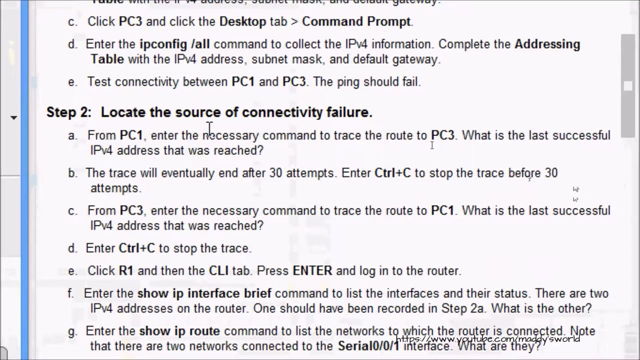 now we are going to ping from this pc1 to pc3. so coming to pc1 command prompt, here we are going to ping to pc3 ip address. last, We are getting herself uh destination host unreachable. now we will come to step two: locate the source of connectivity failure. 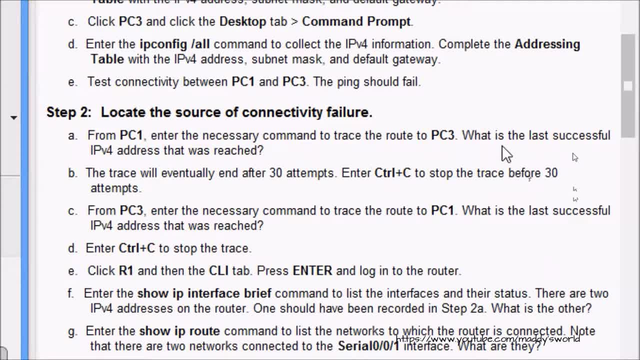 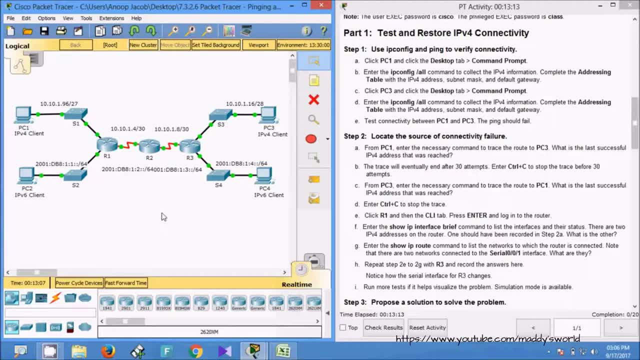 necessary command to trace the root to pc3. what is the last successful ipv4 access that was reached? all right, we will verify that. we will come to pc one. come on, promp unhof gosh. all right, now we are going to open a file server. less than usually answers, so, um, we will press star b. it also gave us the. 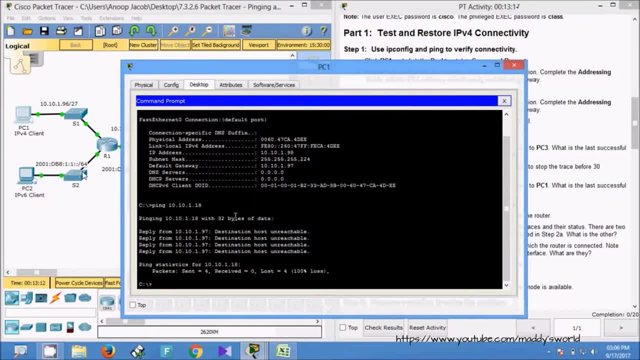 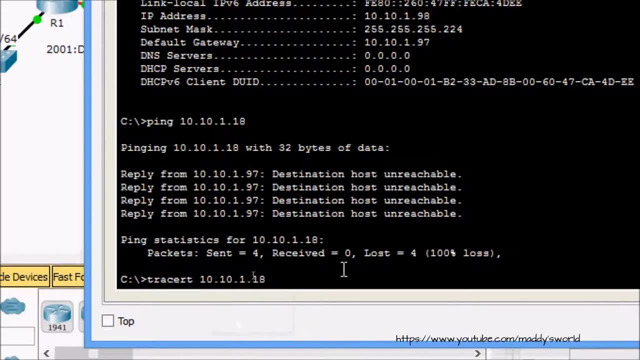 password: theater dot of rambar. and now we have learned how to connect phd, our first holding command. so right now we have two fields. is it possible, uh, pp, c1 command prompt, and i will ninety more praying- to consider one command prompt? and here we are going to give the command tracer and pc3 ip address and we are 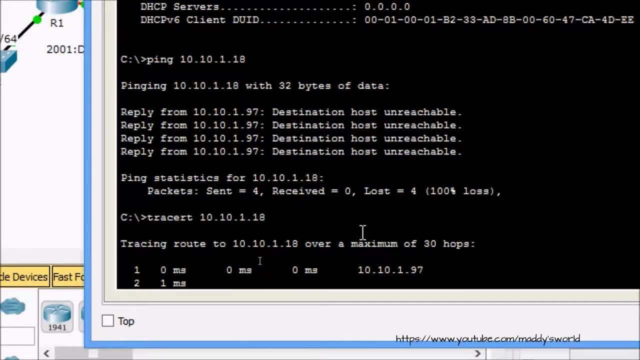 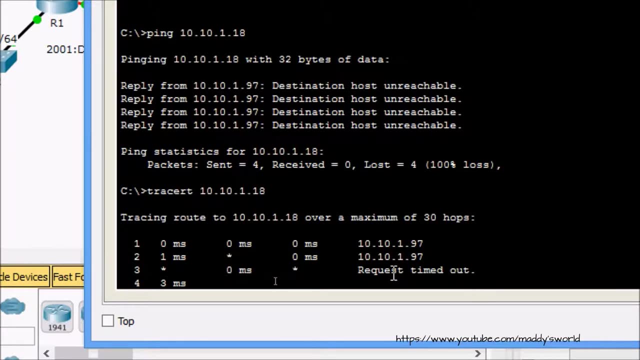 going to press enter. now we go 10.10.1.97, then we are waiting 10.10.1.97, then request timed out. so this is the uh how we can same ip address we are getting. uh. this might be the uh last successful ipv4 address. 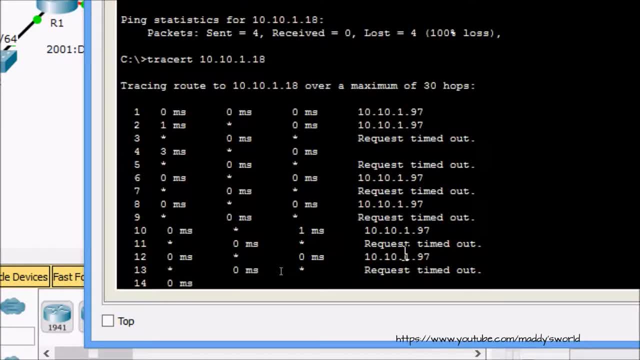 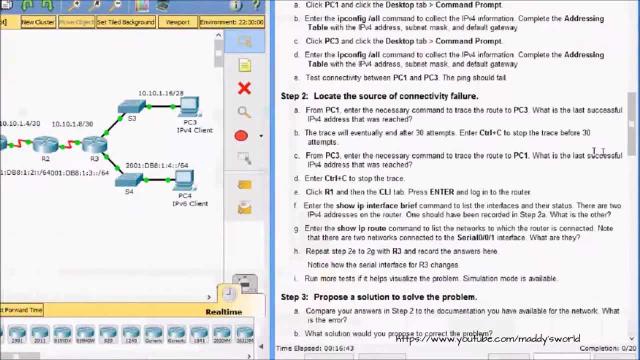 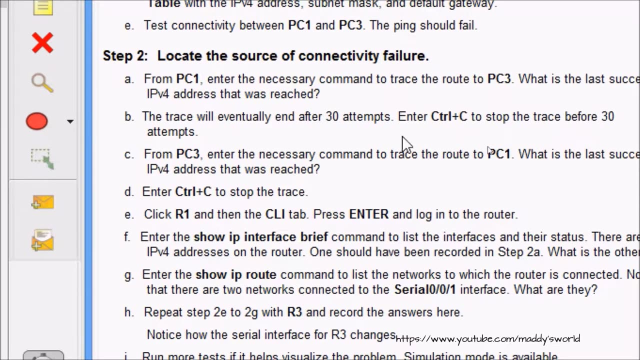 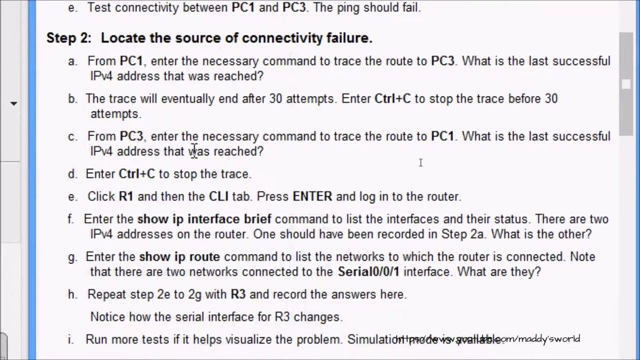 right. here we can see the last successful ipv4 address: uh, that was reached is a 10.10.1.97. next is: the trace will eventually end. after 30 attempts, enter ctrl c to stop the trace. before 30 attempts, right then. next is from pc3. enter the necessary command to trace the route to pc1. 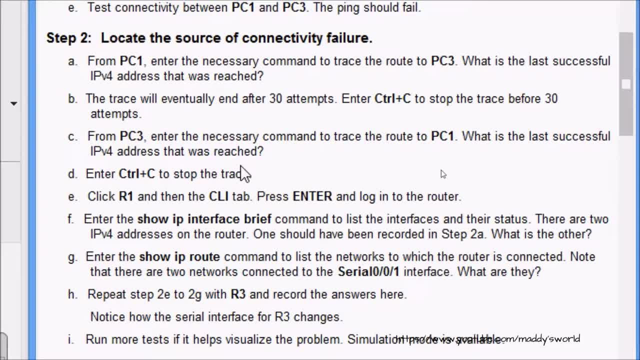 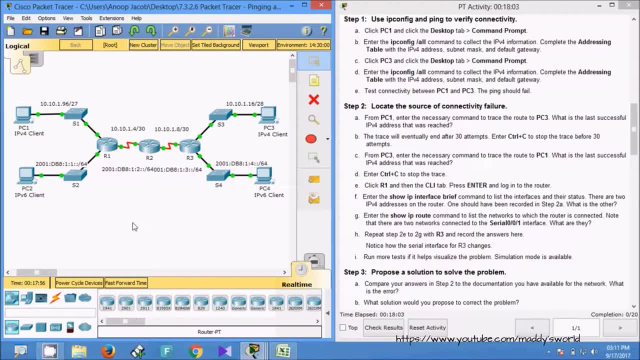 what is the last successful ipv4 address that was reached right? we will try that. enter ctrl c to stop the trace right. we will try this now before going to that. uh, in the previous tracer we have seen the last successful ipv4 address was reached uh 10.10.1.97, and here we can see that ip address. 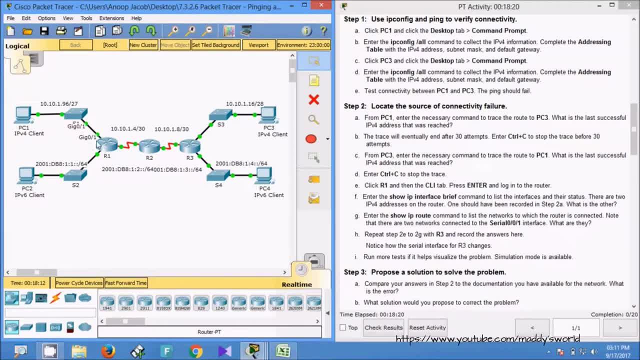 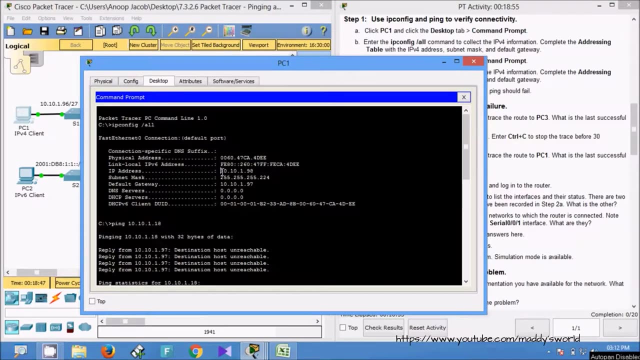 is is the address of this interface, a gigabit 301 on this device r1. now we will give the tracer command from pc3 to pc1. before that we will get the ip address of pc1. here is that. i'm going to copy this at: 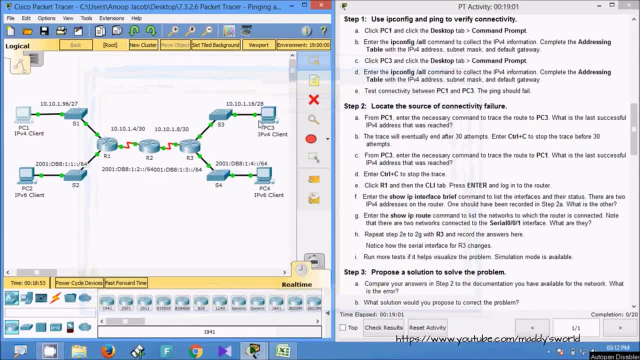 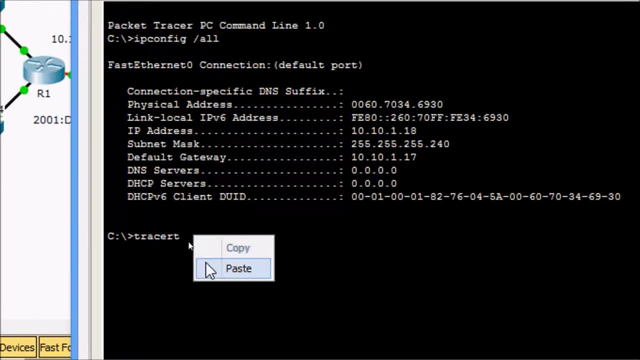 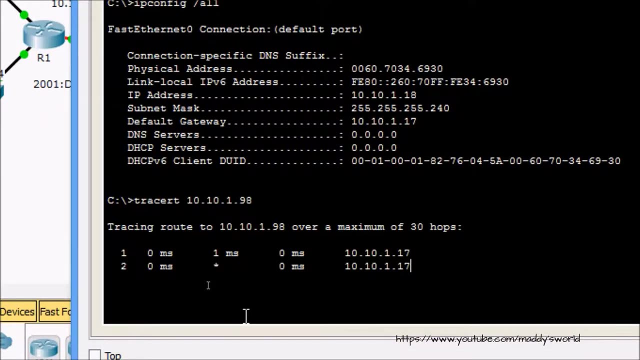 address. right now we will come to pc3 command prompt. here we are going to give tracer and the pc1 ip address right. so here we get the ip address 10.10.1.17. so this will be the last uh successful ipv4 access reach. 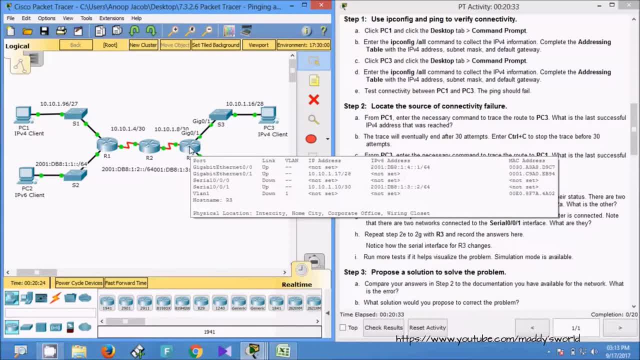 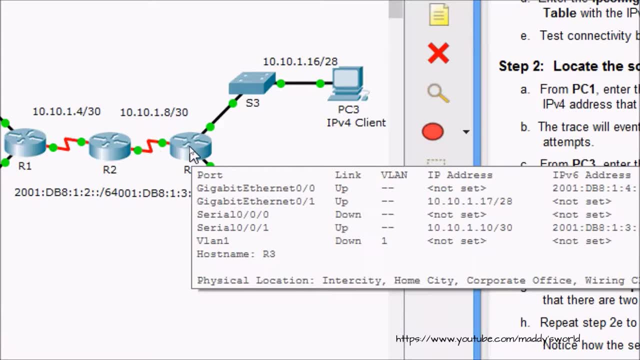 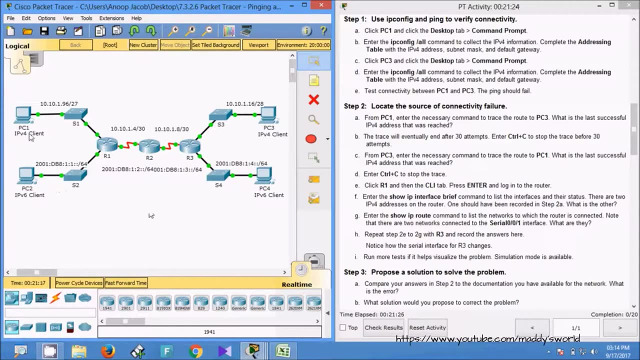 that is 10.10.1.17. here we can see this ip address is of a gigabit third zero slash one on interface, i mean on the device r3. yes, so when we trace from pc1 to pc3 we have seen the package. 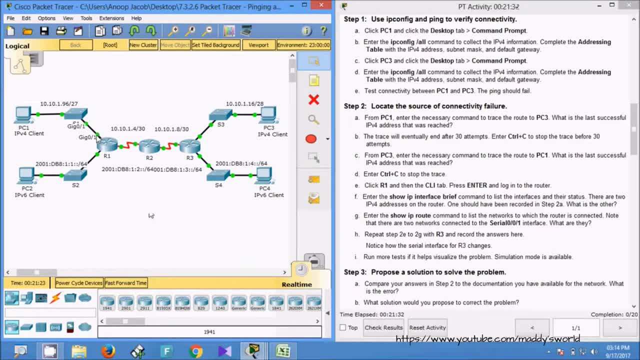 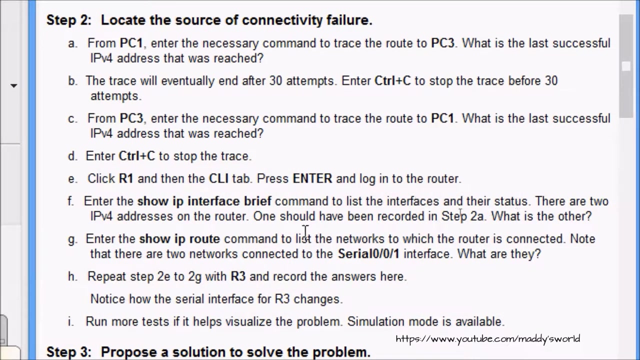 reached from pc1- uh till this r1 interface, a gigabit third zero slash one, and from pc3 to pc1, the packet to reach it from uh till this interface, a gigabit 130 slash one on r3. now we will come to the next. click r1 and then the cli tab, press enter and login to the router. 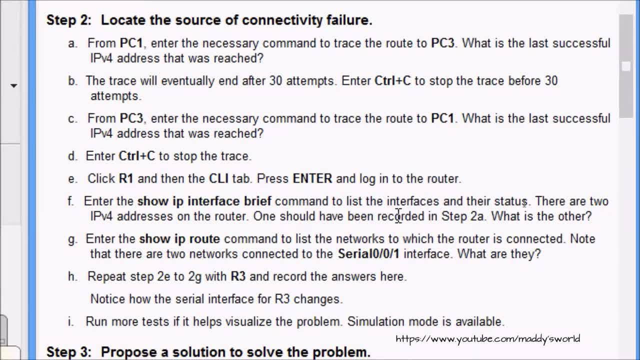 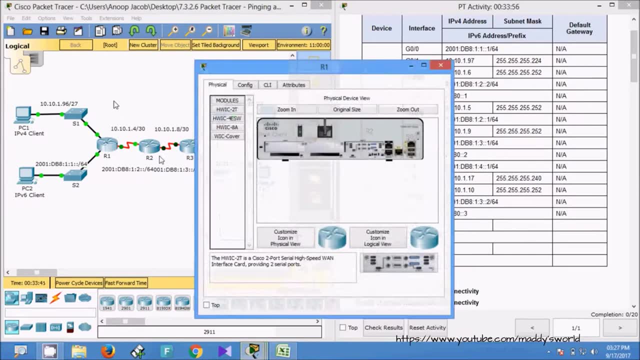 enter the show ip interface brief command to list the interfaces and their status. there are two ipv4 addresses on the router. one should have been recorded in step 2a a. what is the other, right? we will verify that. coming to r1 cli: right, we will press enter. 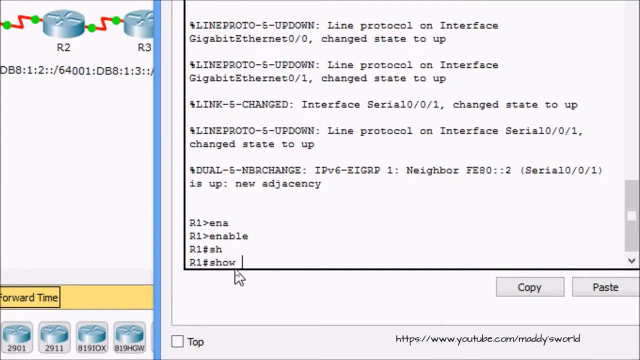 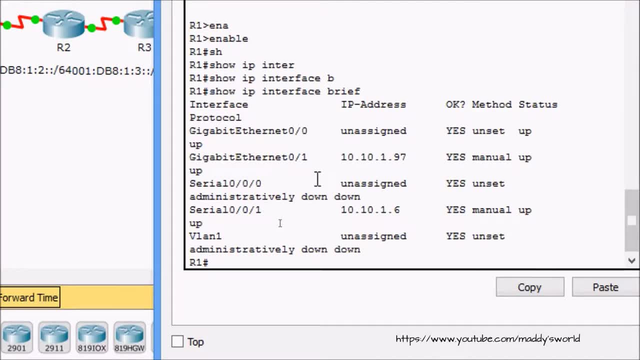 enable. now we are going to give the command show ip interface brief, and here we can see two ipv4 addresses: 10.10.1.97. yes, this address we have been recorded in our spreadsheet as a pc1, a default gateway, and this is the address: yes, 10.10.1.6. 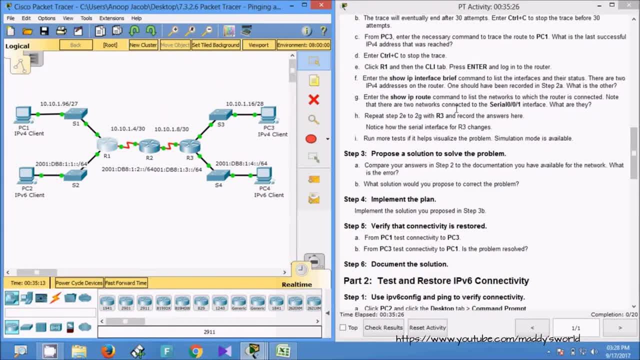 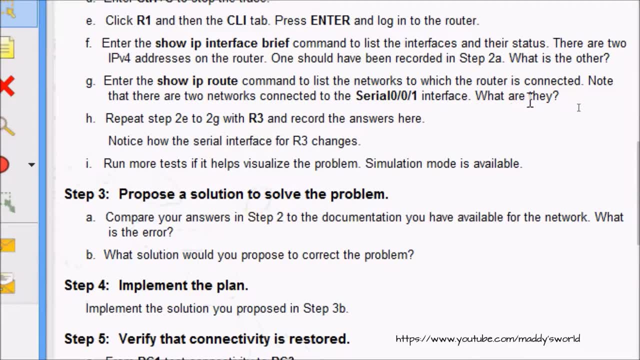 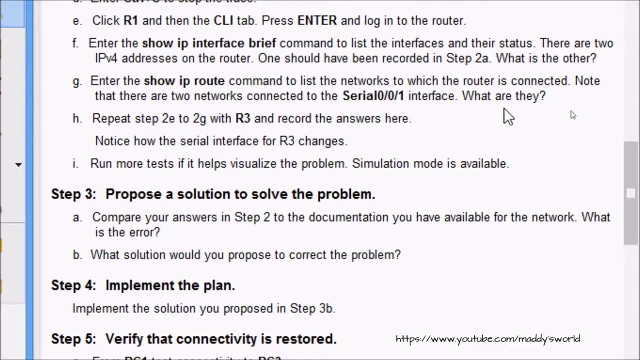 now we will go to g, enter the show ip root command to list the networks to which the router is connected. note that there are two networks connected to the serial 0 0 0, 1 interface. what are they right? we will verify that. coming to r1. so here we are going to. 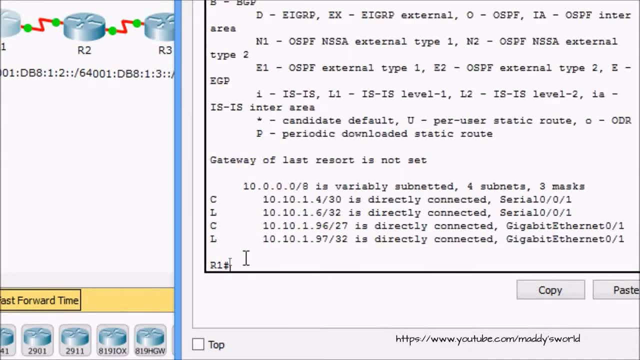 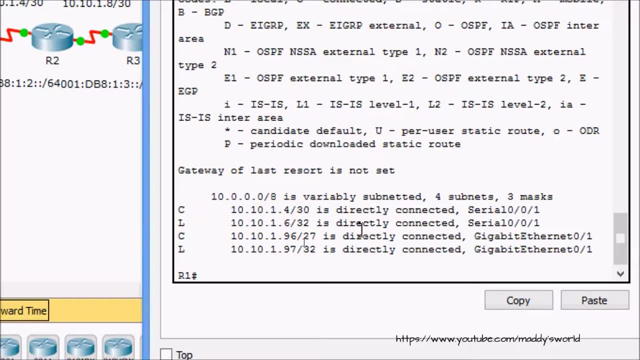 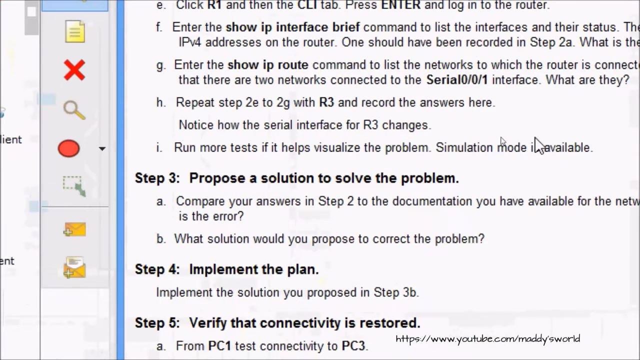 give show ip root. here we can see, here we can see: there are two networks connected to the serial 0 0 0 1 interface. we can see that 10.10.1.4 slash 30 and 10.10.1.6 slash 32. now we will come to h. 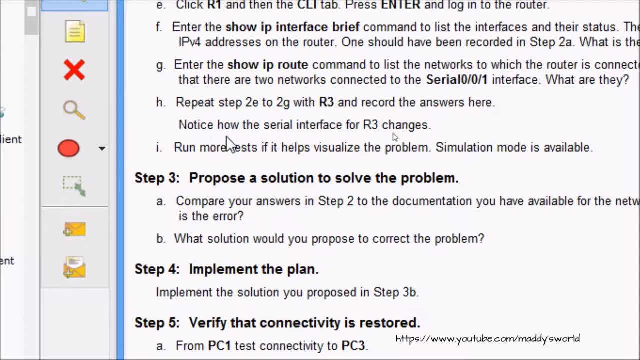 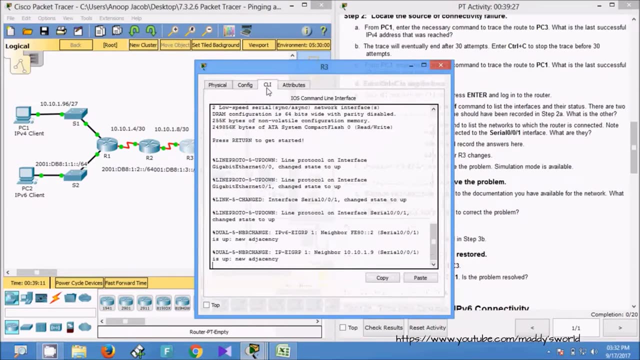 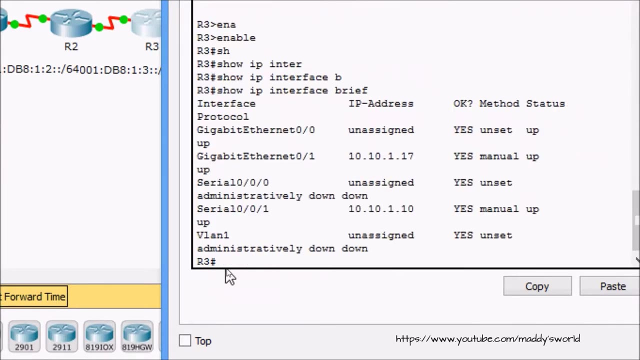 with r3 and to record the answers here. notice how the serial interfaces for r3 changes. run more tests. if it helps visualize the problem, simulation mode is available right, so we will do it on r3. now, coming to s3, cli right enable. first we are going to give a show ip interface brief, and here we can. 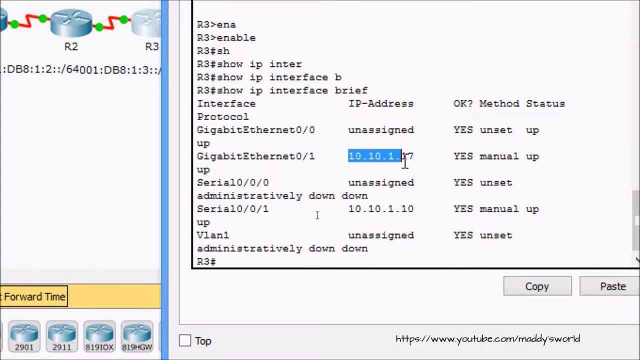 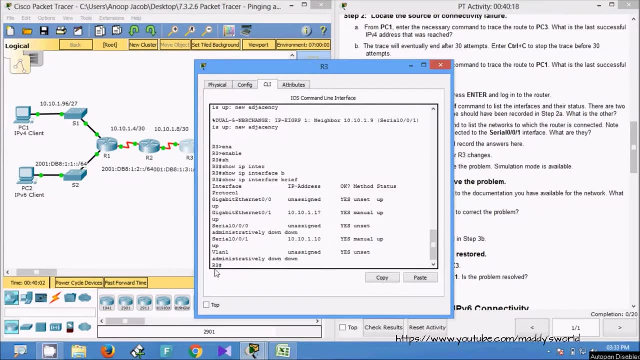 see the address 10.10.1.17. this is the address been noted in our spreadsheet. this is the default as a default gateway of pc3, and here we can see the other address, 10.10.1.10. next we will give the command show ip root. 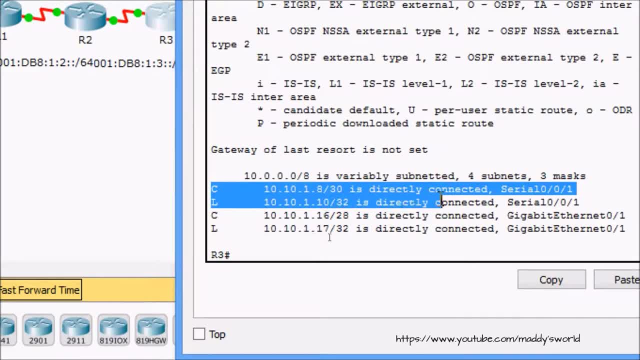 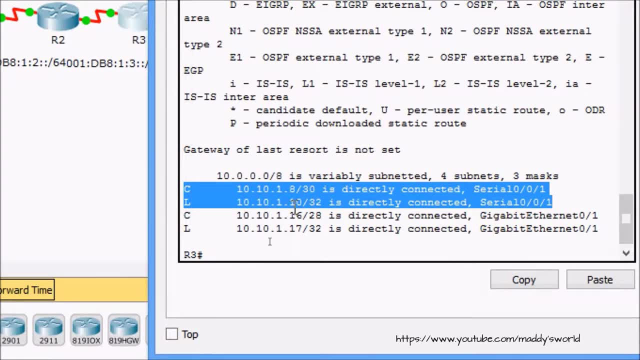 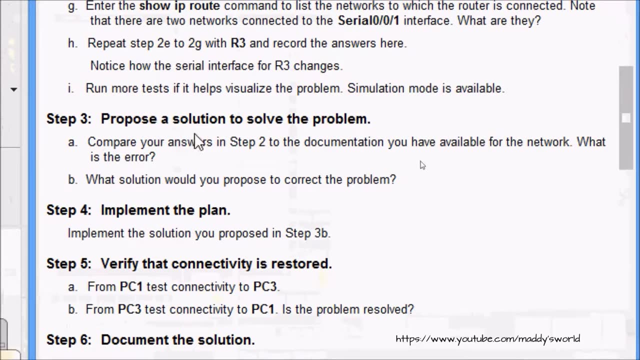 and here we can see the two addresses, which is connected to serial 0 0 0 1, that is, a 10.10.1 dot 8 slash 30 and 10.10.1.10 slash 32.. now we will come to a step 3: propose a solution to. 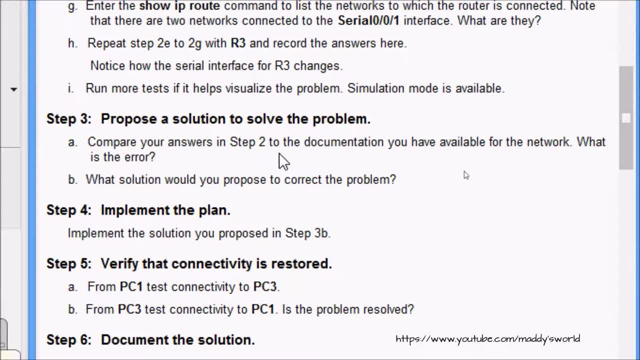 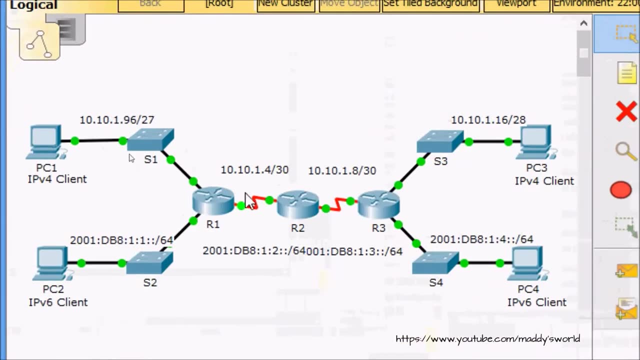 solve the problem. compare your answers in step 2 to the documentation you have available for the network. what is the error and what solution would you propose to correct the problem? right, we will check this now. okay, we will check from the topology so it will be more easier here. here we can. 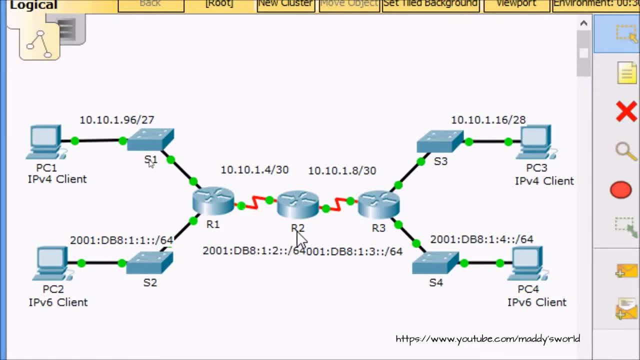 see the network in between the router r1 and r2. here the used network is a 10.10.1.4 slash 30. here the cidr is 30. that means here we have two usable ip address, that is, a 10.10.1.5 and 10.10.1.6. so 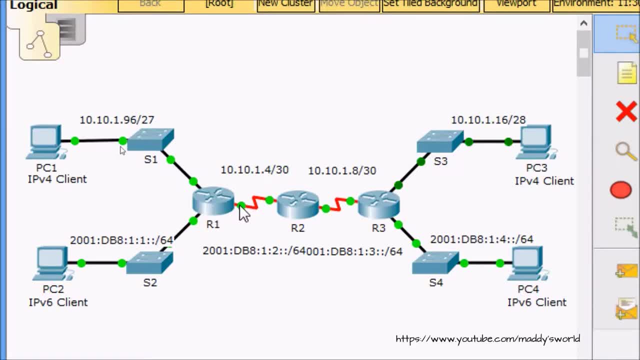 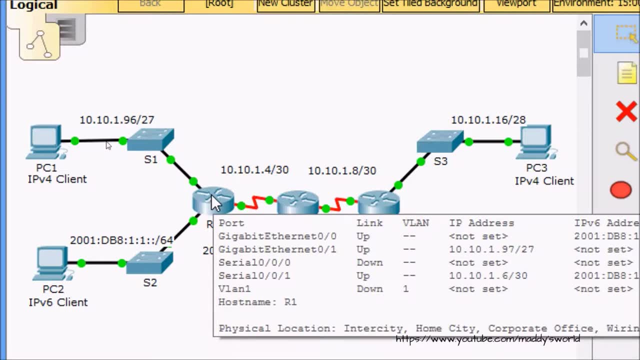 this is two address can be used. so here on r1 for this interface. so that is serial 0, slash 0, slash 1. the ip address, that is the 10.10.1.6. okay, it's correct. so obviously the ip address for this. 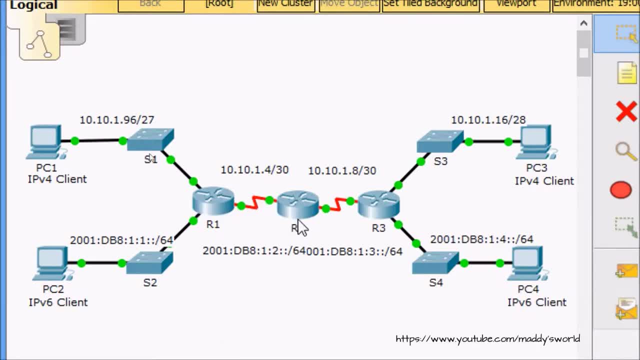 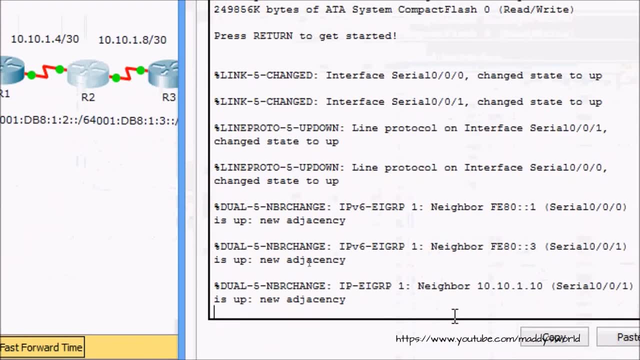 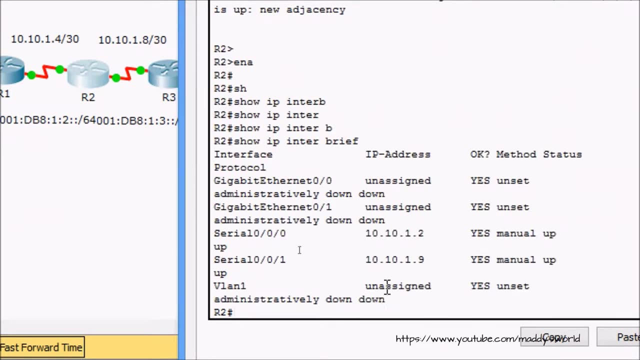 interface, that is, cdl 0 slash 0, slash 0 on r2 should be 10.10.1.5. so we have to verify that. coming to cli, enable show ip interface brief. here we can see that yes, so here the ip address of this. 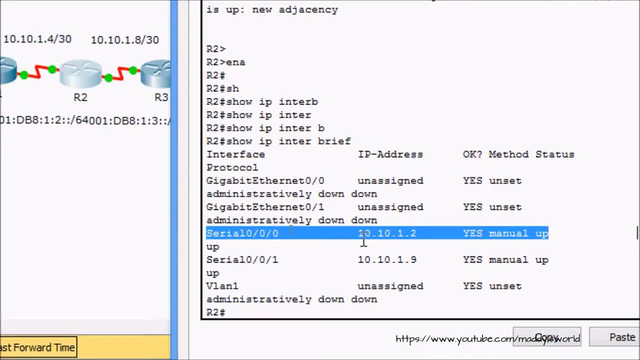 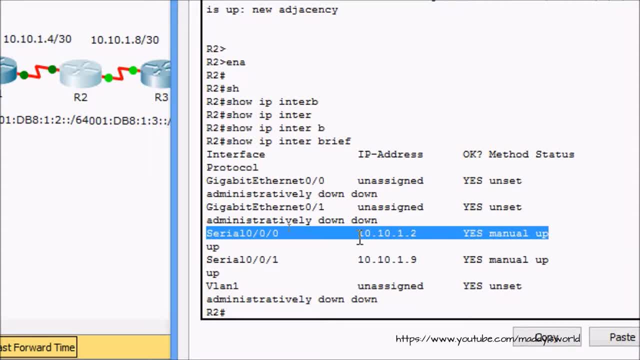 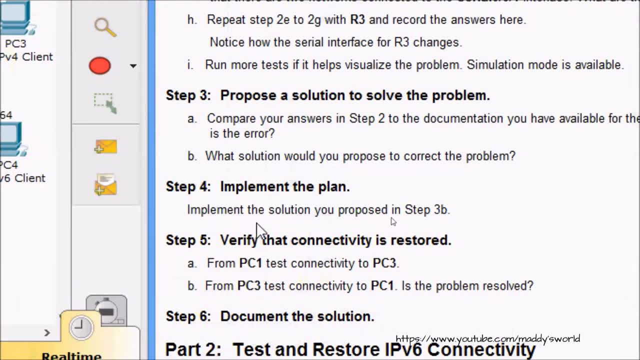 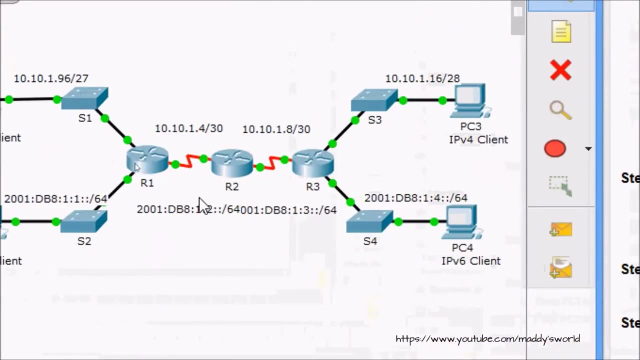 to change this address. we have to change this address of this interface: cdl 0- slash 0, slash 0. now we will come to step 4. implement the plan. implement the solution you proposed in step 3b. right here, the solution is: we must change the ip address of this interface: cdl 0- slash 0, slash 0. 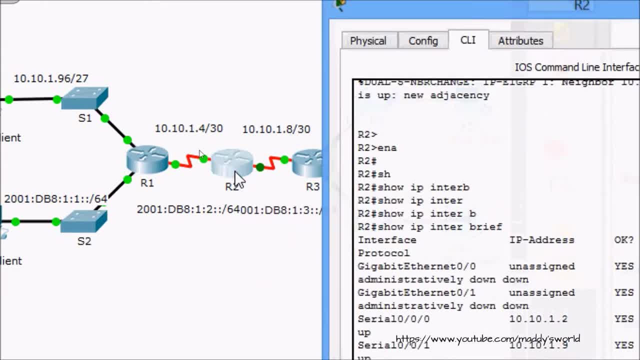 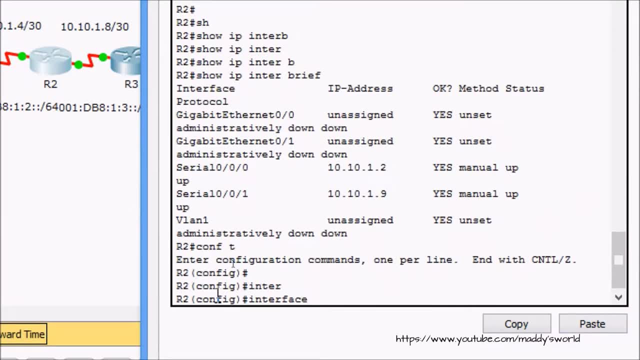 on r2: right, we will change that. coming to cli: configure terminal- configure terminal, configure terminal. we have to go to the interface: uh cdl 0, slash 0, slash 0, and we are going to set. we have to go to the interface: uh cdl 0, slash 0, slash 0, and we are going to set. 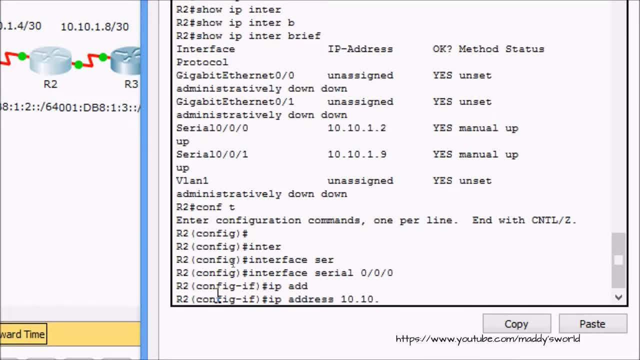 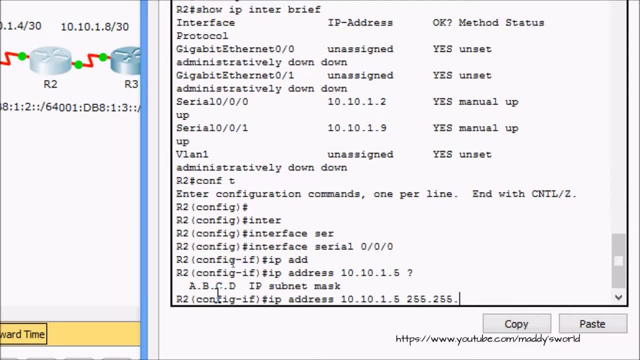 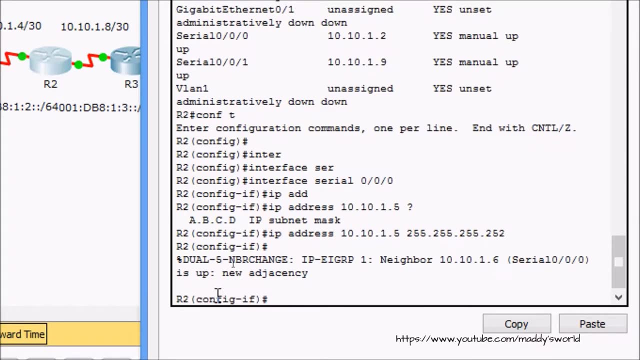 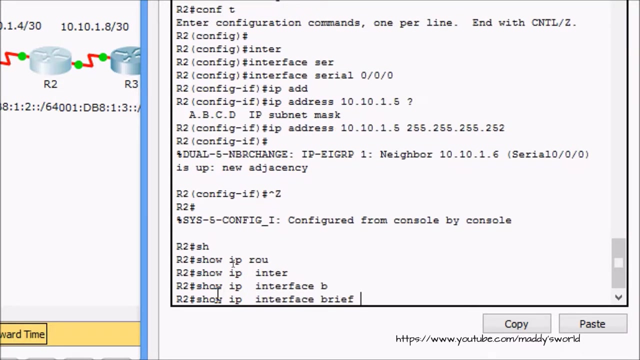 the ip address, uh, 10.10.1.5. and here we have to specify the subject mask, that is 255.255.255.252. yes, and now we will cross check it to show ip. oops show ip. yes, and now we will cross check it to show ip. oops, show ip. 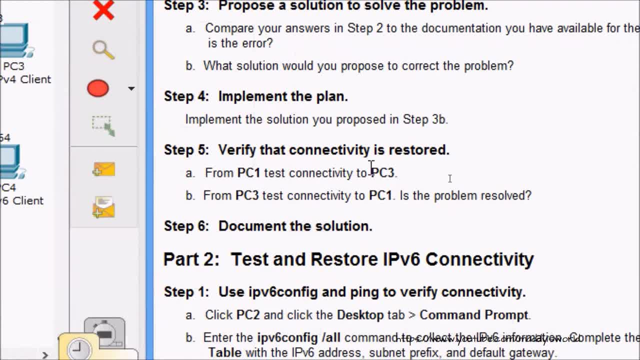 now we will come to step five. verify that. now we will come to step five. verify that. now we will come to step five. verify that connectivity is a restored connectivity is a restored connectivity is a restored from. pc1 test connectivity to pc3 from. from pc1: test connectivity to pc3 from. 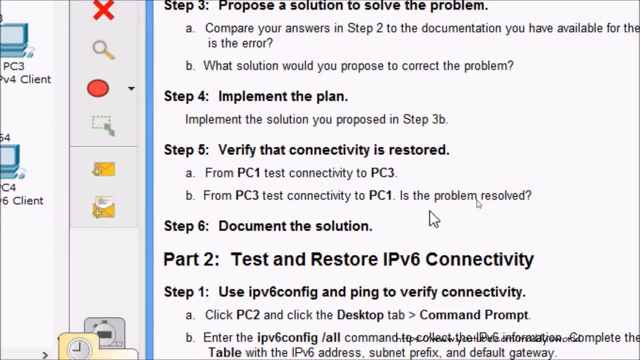 from pc1 test connectivity to pc3. from pc3 test. connectivity to pc1. is the pc3 test. connectivity to pc1: is the pc3 test. connectivity to pc1. is the problem resolved, problem resolved, problem resolved. uh, we have to verify that. coming to pc: 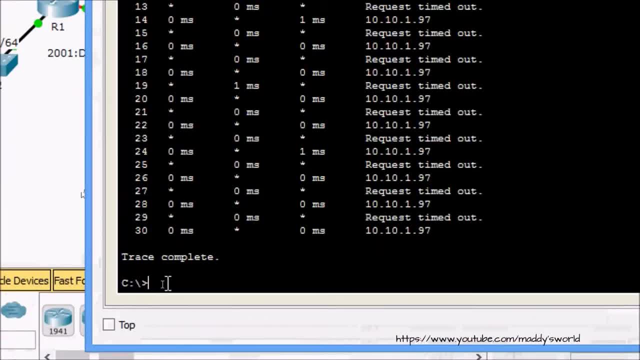 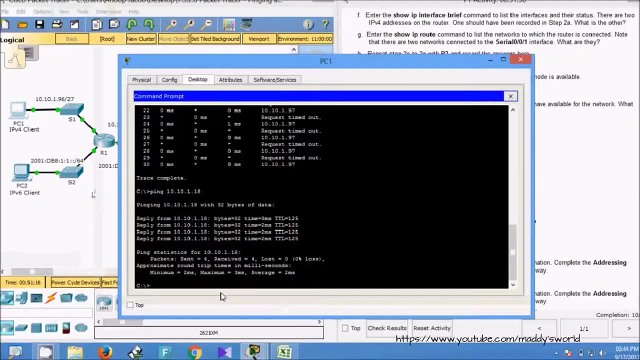 uh, we have to verify that. coming to pc. uh, we have to verify that. coming to pc. one command prompt now. we will ping to one command prompt now. we will ping to one command prompt. now we will ping to pc3, pc3. yes, here it is. yes, we are getting the replay. now we will go to pc3. 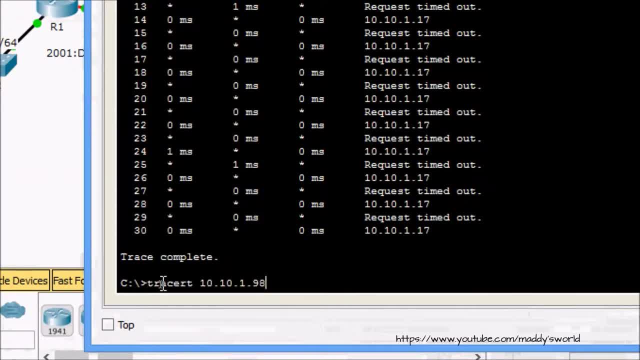 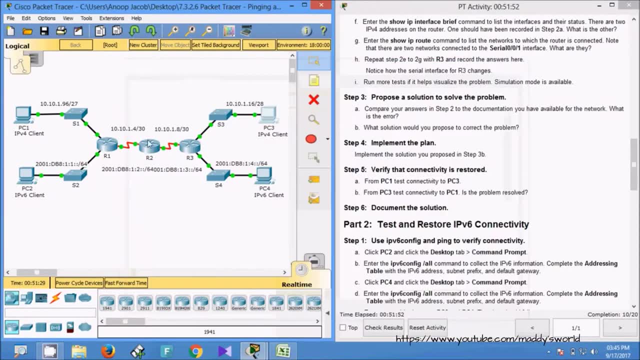 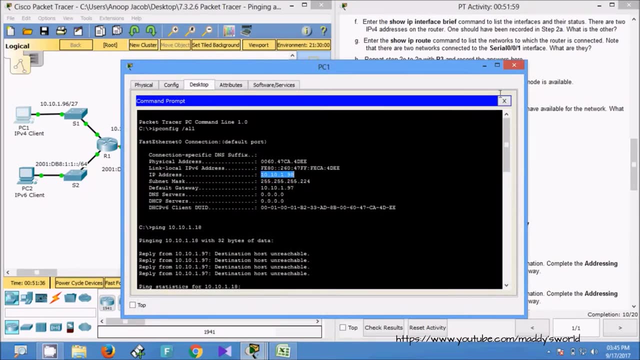 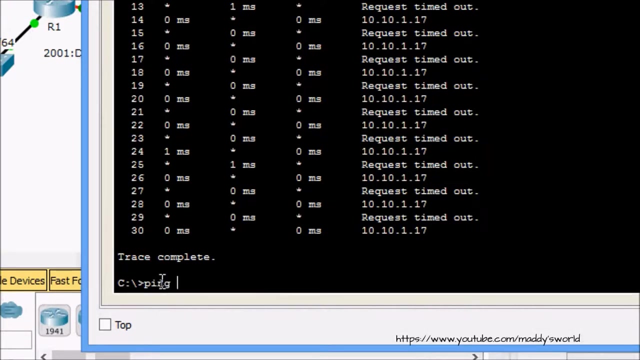 yes, command prompt. we are going to ping 2. right, so we will get the ip address of a pc1 command prompt. here we can see. i'm going to copy that. coming to pc3 command prompt: here we will give a ping. yes, we are getting the replay. 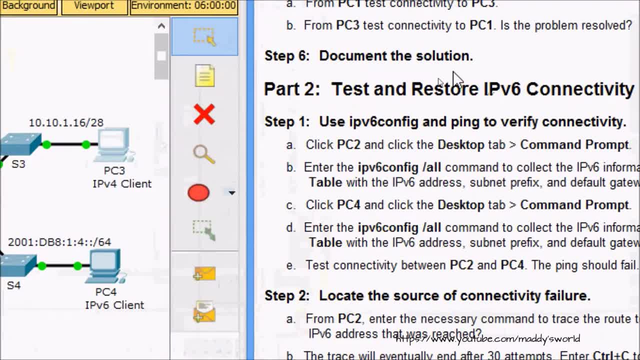 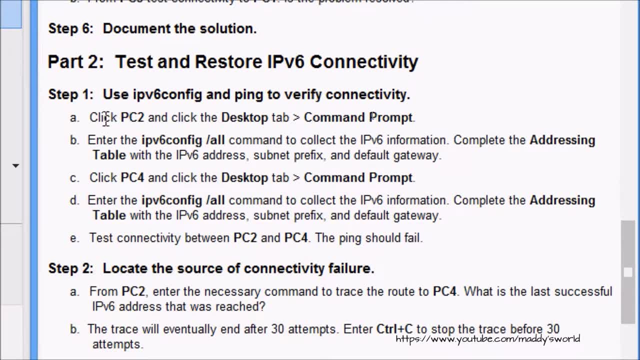 now we will come to step six here. document the solution. anyway, we implement the solution here. now we will come to party two. test under restore ipv6 connectivity, use ipv6 config and ping. to verify connectivity: click pc2 and click the desktop tab command prompt. we have to give the command ipv6. 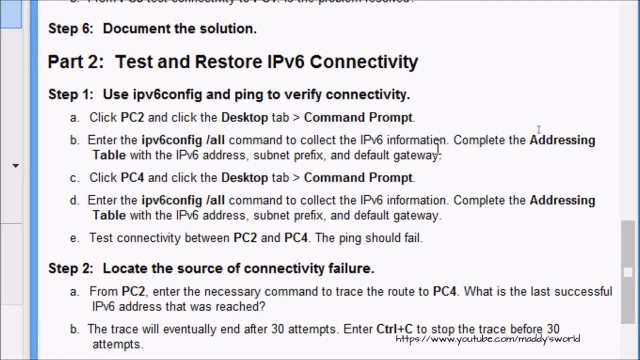 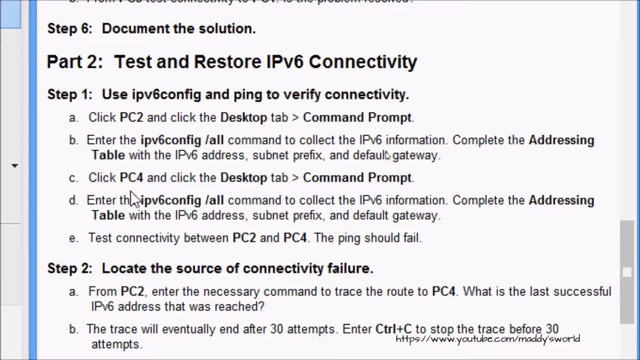 config slash all command to collect the ipv6 information. complete the addressing table with the ipv6 address, subnet prefix and default gateway. also, we have to get the information from pc4. give ipv6 config space slash all command to collect the ipv6 information. complete the addressing table with the ipv6 such as sub prefix and default gateway. test connectivity between pc2. 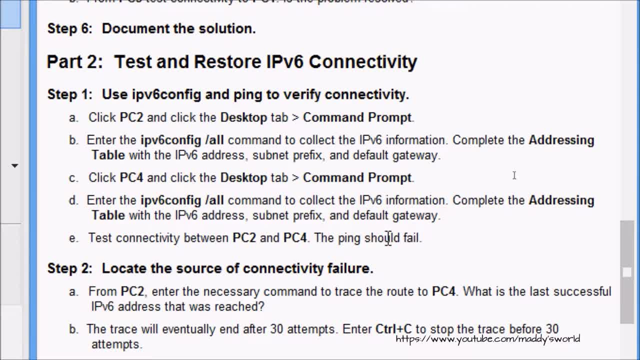 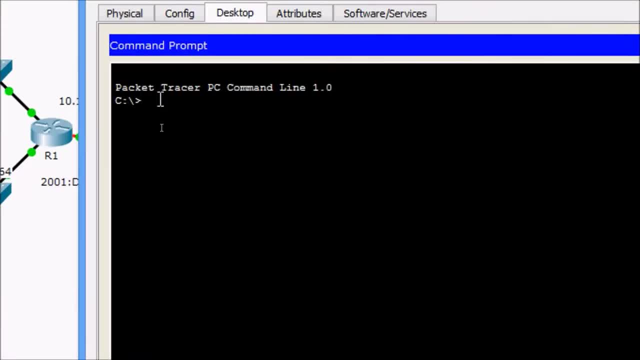 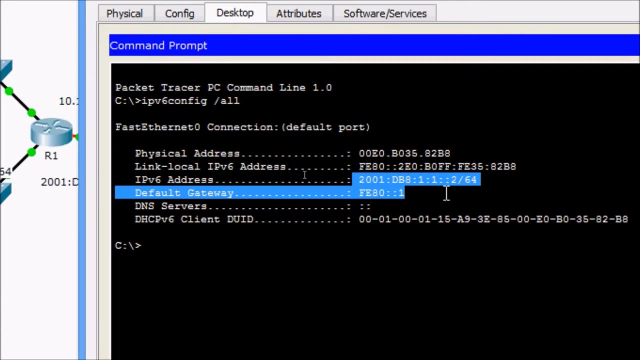 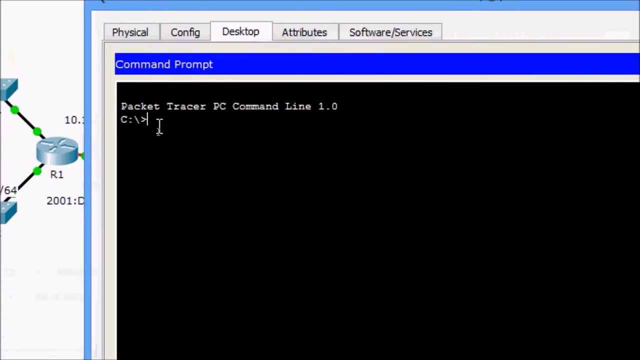 and pc4. the ping should fail. right, we will do this. now, coming to pc2 command prompt, here we are going to give ipv6 config all, and here we can see the address, ipv6 address. then default gateway: right, and we will come to pc4 desktop command prompt, and here we are going to give ipv6. 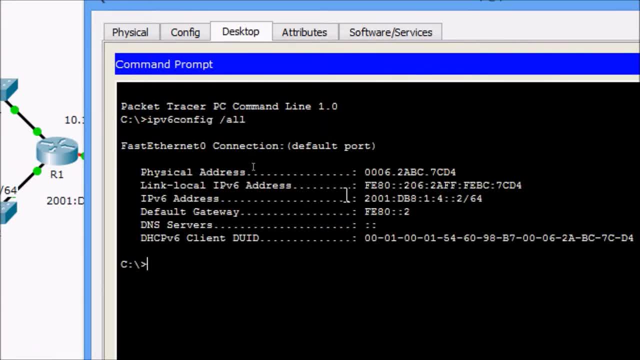 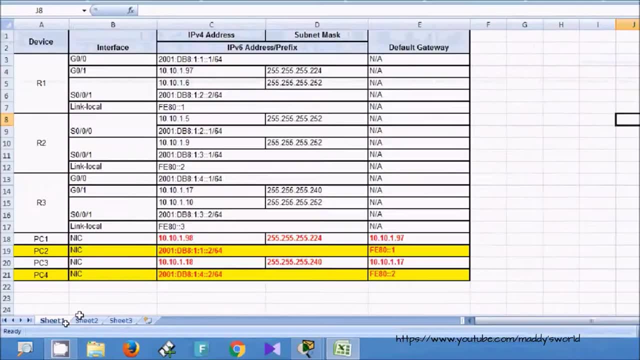 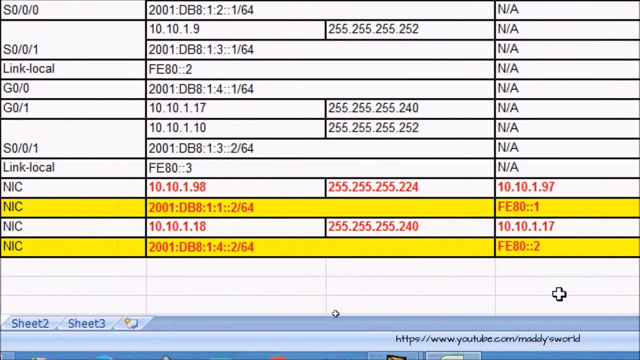 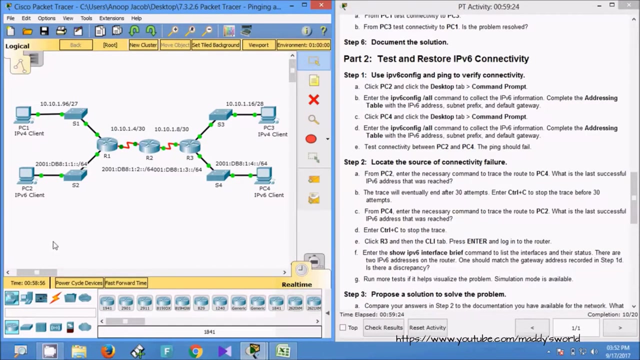 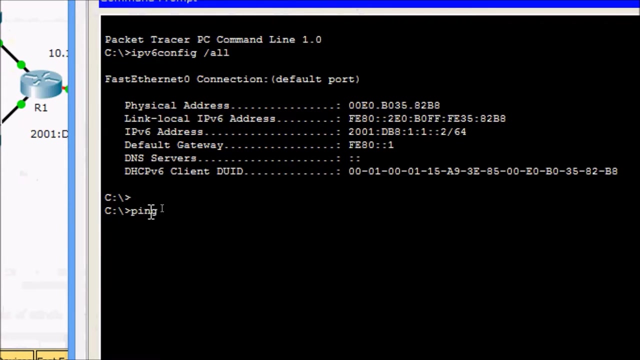 config space all and here we can see the details. okay, we will update this information into our addressing table. yes, here we can see the details updated in our addressing table. pc2 and pc4: ipv6 address and default gateway. now we will ping from pc2 to this pc4. so, coming to pc2 command prompt, here we are going to. 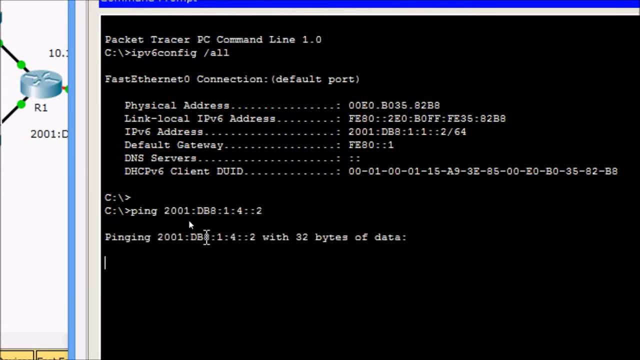 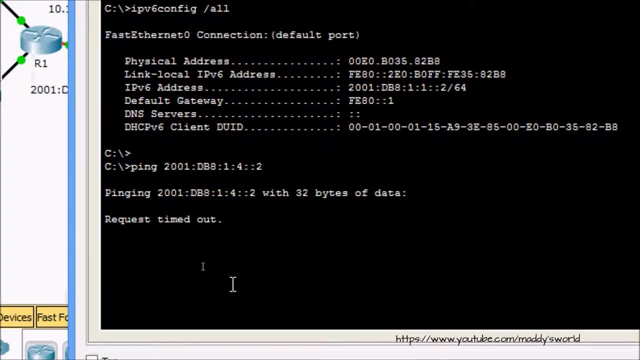 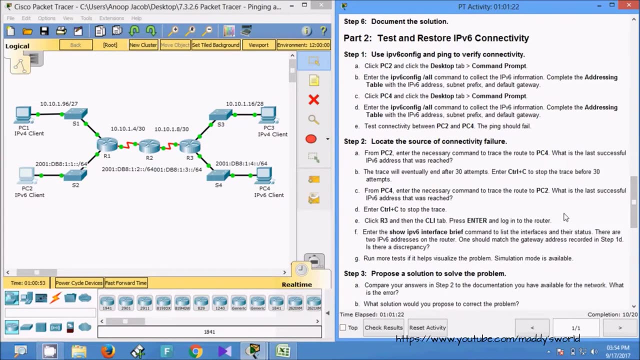 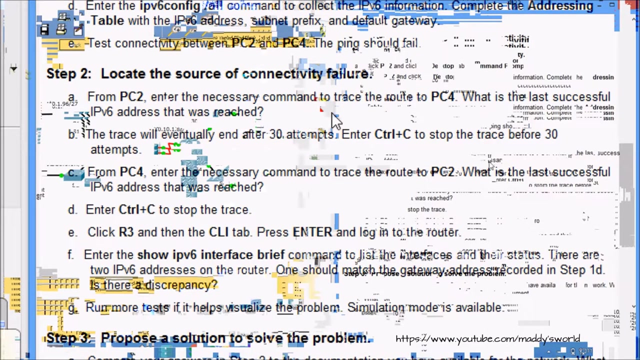 give the ipv6 address of pc4. we are waiting for the replay request timed out. here we can see the ping is unsuccessful. now we will come to step 2: locate the source of connectivity failure from pc to enter the necessary command to trace the route to pc4. what is the last successful ipv6 address that was reached? 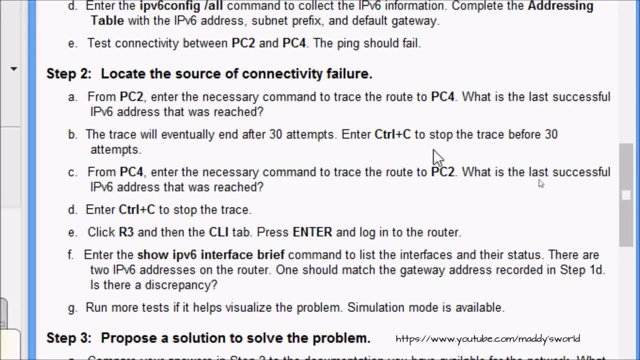 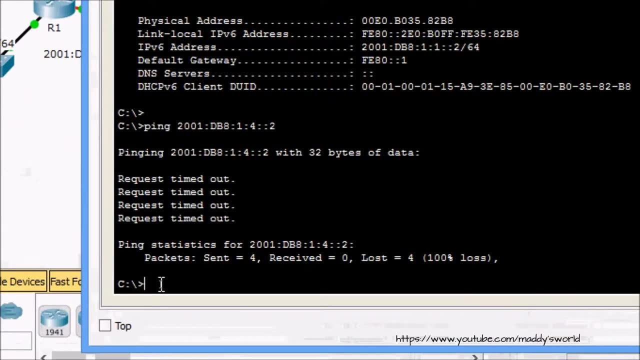 and the trace will eventually end. after 30 attempts, enter ctrl c to stop the trace. before 30 attempts: right, we will trace from this pc to pc4. we will give the traced command on pc2 a pc2 coming to pc2 command prompt. here we are going to give a tracer and the ip address of pc4. 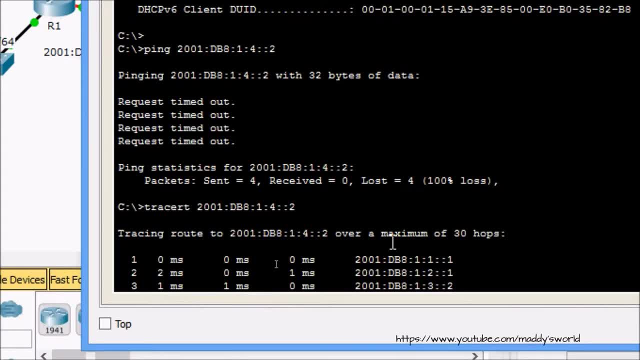 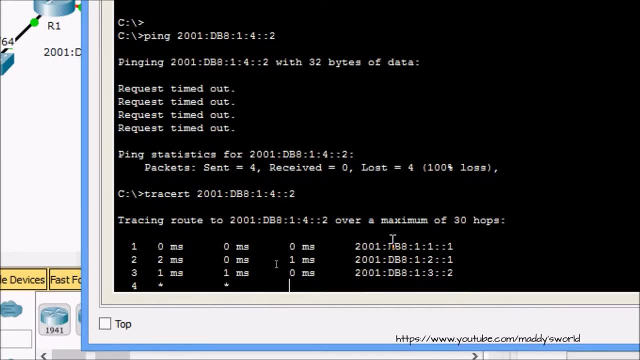 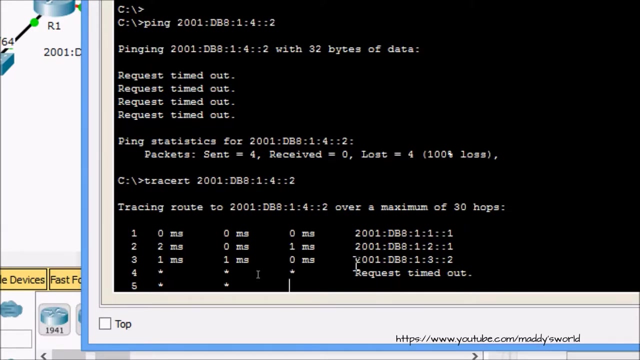 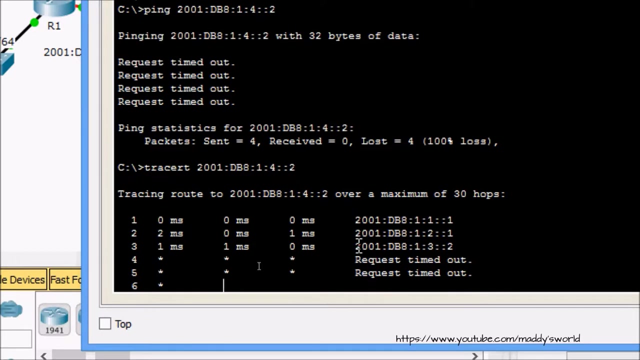 and here we are waiting. here we go to 2001 colon db 8, colon 1, colon 3, double colon 2. so we are waiting for the tracer to request timed out. so here we can see: the last successful ipv6 address reached is a 2001 colon db 8, colon 1, colon 3. 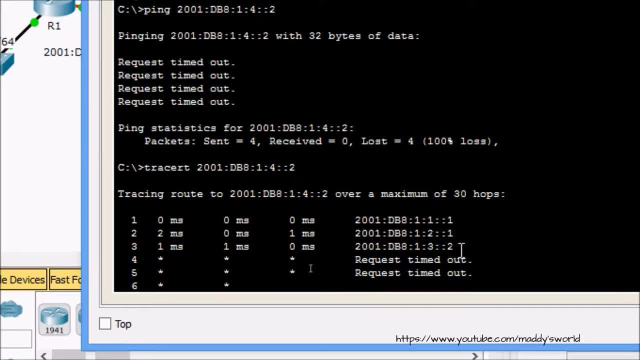 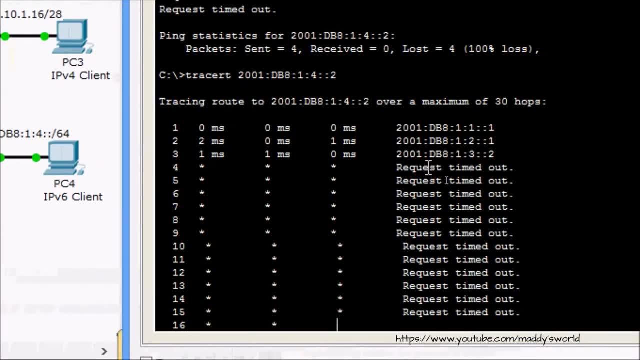 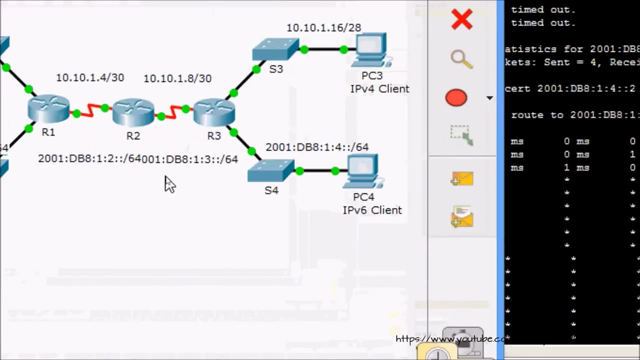 double colon 2: right? yes, so this is the last successful ipv6 address reached is a 2001. this last successful ipv6 v6 address 2001, colon db 8, colon 1, colon 3, double colon 2 is the ip address of this interface. that is serial 0 0 0, 1 on r3. yes, here we can see that. 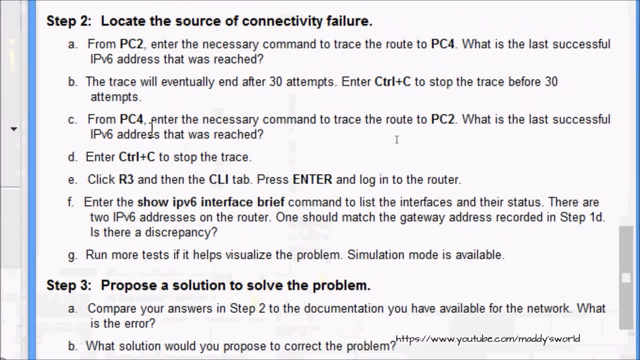 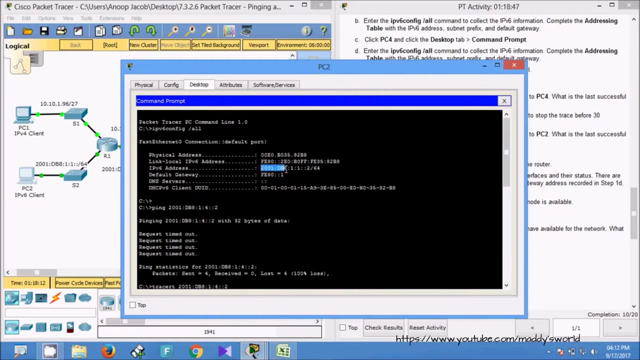 yes, we will come to see from pc4. enter the necessary command to trace the route to pc2. what is the last successful ipv6 address that was reached? yes, we will verify that. enter ctrl c to stop the trace right. first of all, we will get the ipv6 address of pc2. yes, here it is. we will copy this. 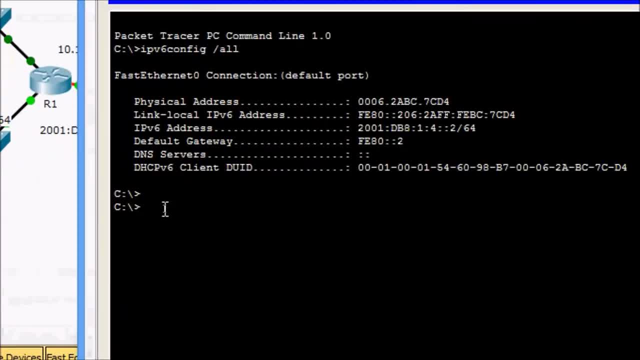 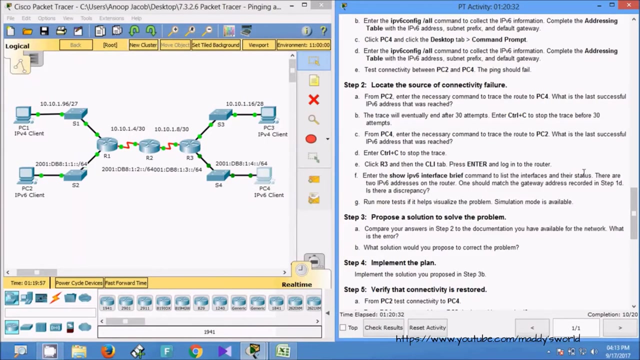 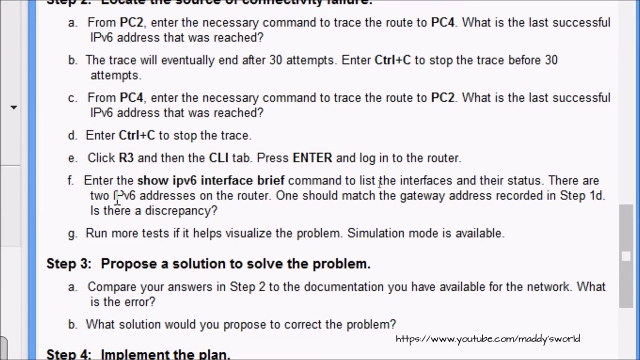 coming to pc4 command prompt, here we are going to give tracer, then ipv6 address of pc2. here we can see that. oh, here we can see no ipv6 access was reached. next is click r3 and then the see l i tab presenter and log into the router, enter the show ipv6 interface brief command to. 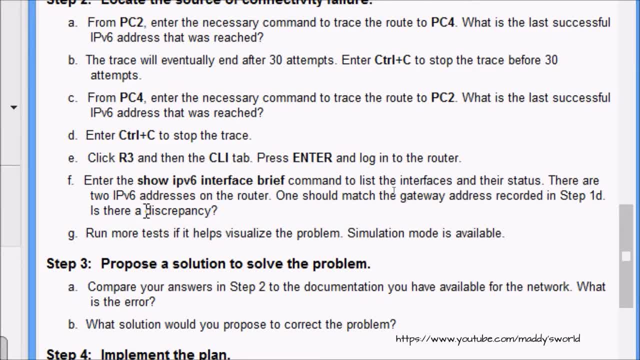 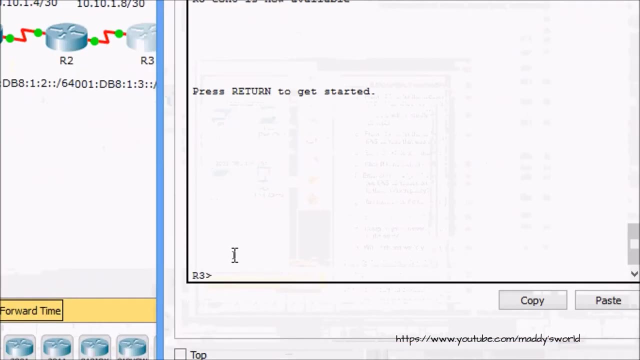 list the interfaces and their status. there are two ipv6 attrass otter. one should match the gateway just recorded in a step 1d. is there a discrepancy? we will see that and more tests. if it helps to visualize the problem, simulation means mode is available. right, we will verify this. now, coming to r3: right, enable, we will give. 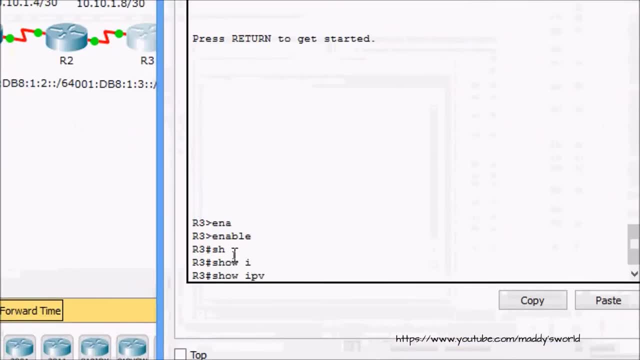 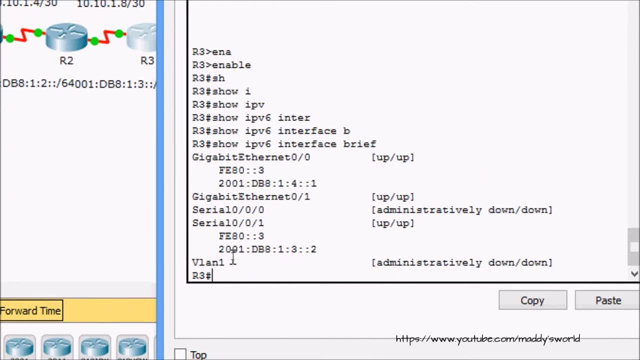 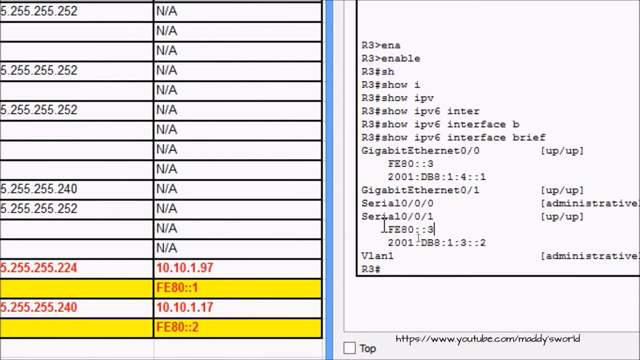 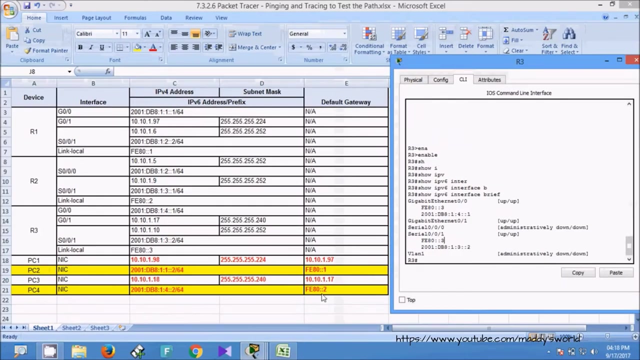 the so command to show IP v6 interface brief, and here we can see the details. ok, now we will compare with our addressing table. here we can see the interface: serial: 0, 0, 0, 1. here we can see F 8, 0, double colon 3. but we given the 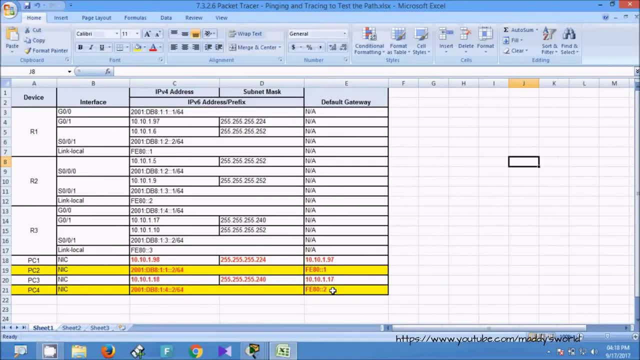 default gateway as F 8 0 double colon 2. so that should be the default gateway. so we can see it as F 8 0 double colon 3, so that. so that should be the default gateway. so we can see it as F 8 0 double colon 2, so that. 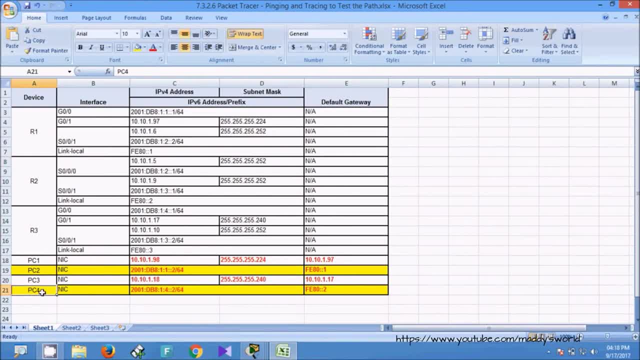 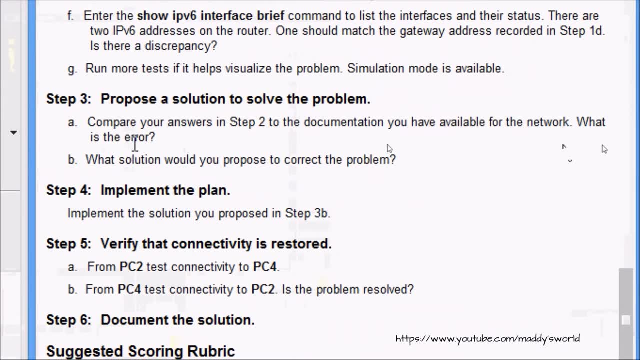 be double colon three, so the pc4 default gateway. we must change. so here is the problem. now we will come to step three. propose a solution to solve the problem. compare your answers in step two to the documentation you have available for the network. what is the error? yes, just now, we have. 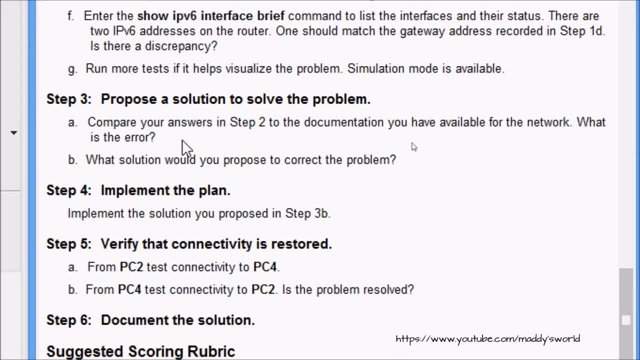 seen that the pc4 is using the wrong default gateway configuration. so we must change that. yes, what solution would you propose to correct the problem? obviously we must change and we must configure pc4 with the correct default gateway address, that is fe80, double, colon three. now we 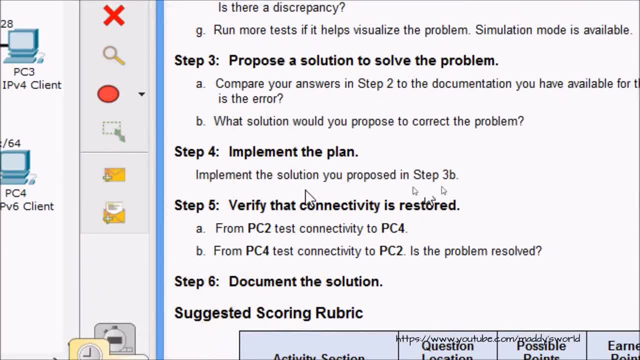 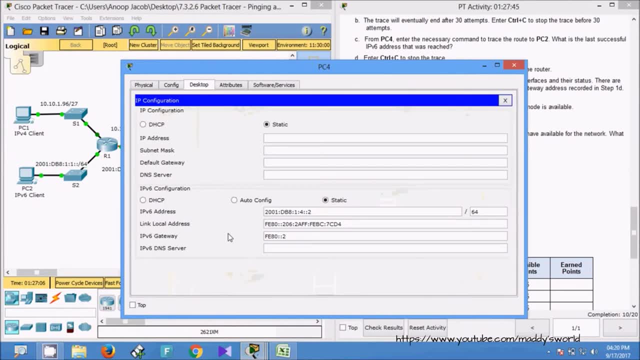 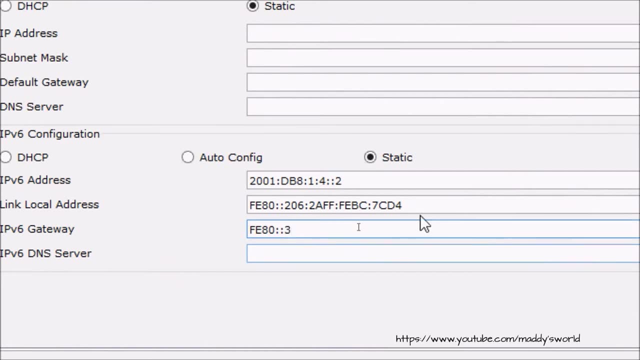 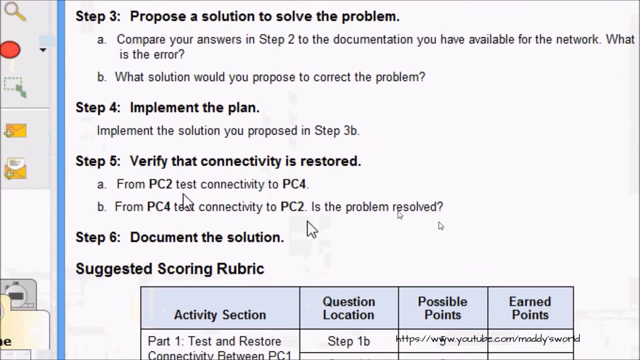 will come to a step four. implement the plan. implement the solution you proposed in step 3b. right, we must change this pcb uh ipv6 default gateway. here we have to give a fe80 zero, double colon three. yes, now we will come to step five. verify that connectivity is a restart from pc2 test. 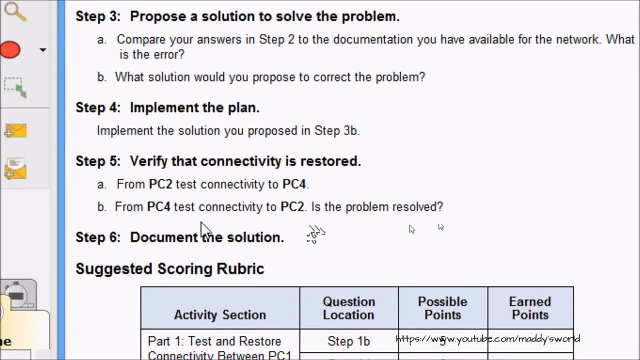 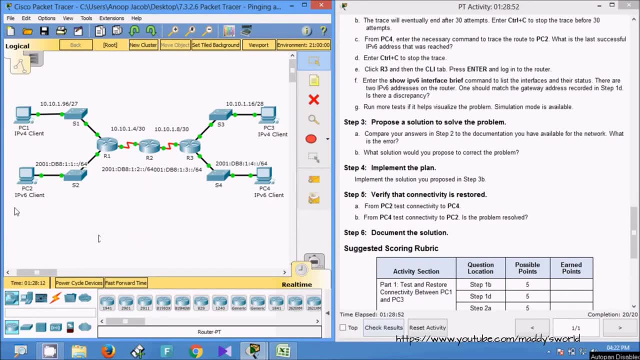 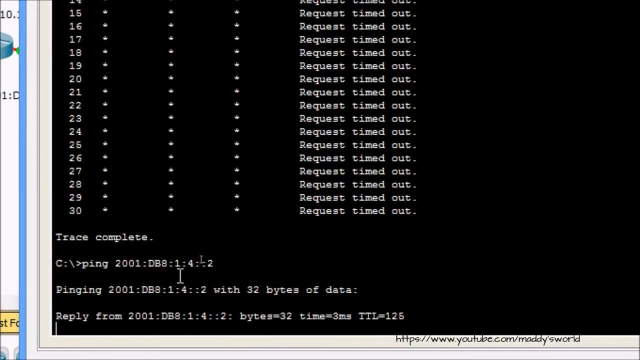 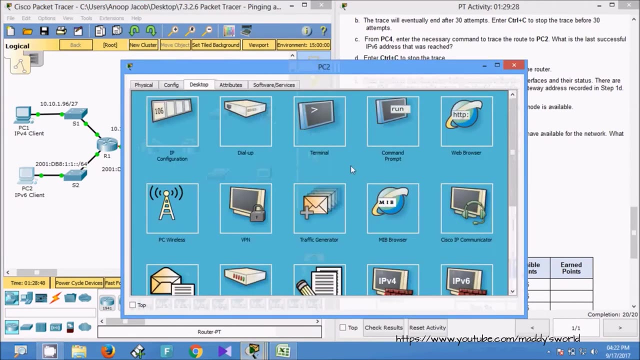 connectivity to pc4 also from pc4 test connectivity to pc2. is the problem resolved? we will verify that now. first of all, we will ping from pc2 to pc4. so here is that thing. yes, we are getting the replay. now we will ping from pc4 to pc2. before that, we will get the. 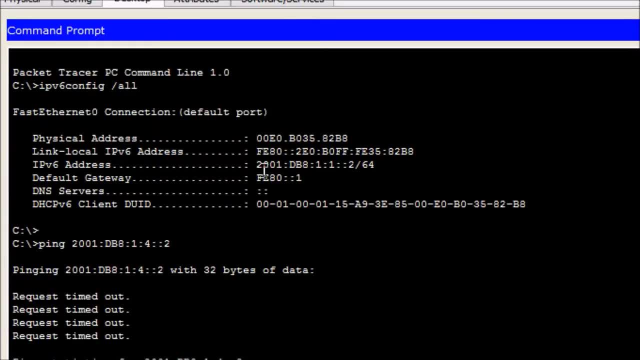 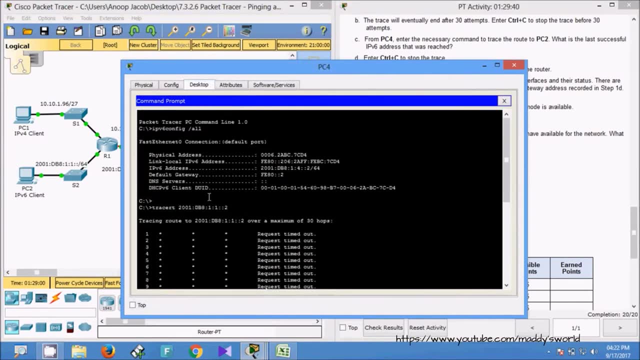 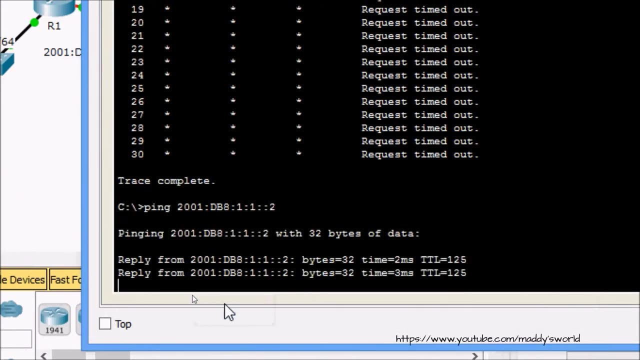 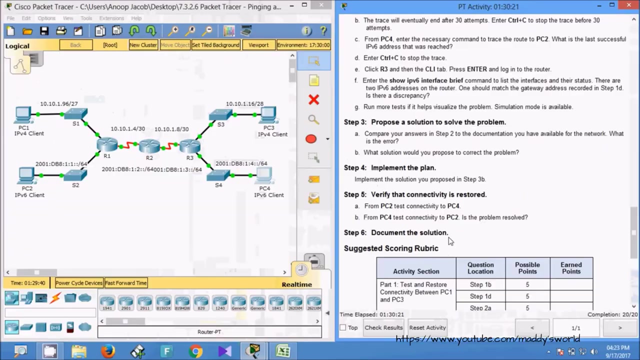 ip address of pc2. yes, here it is. we will copy this address right. coming to pc4 command prompt, here we are going to give ipv6 address of pc2. yes, we are getting the replay. and so here is our last step. document the solution. right, so we implemented the solution. 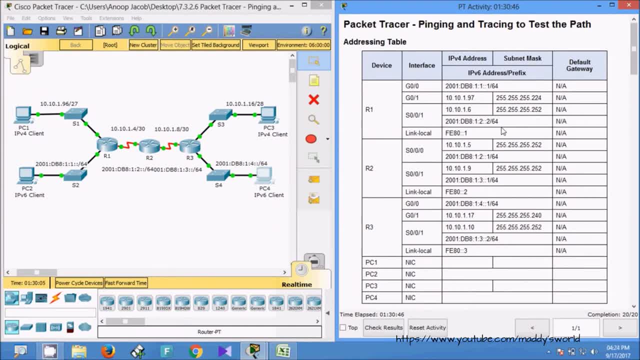 well, friends, that's all in this packet tracer activity, pinging and the tracing to test the path, and in this activity we have seen how to gather the information. also, we have seen ping and trace using ipv4 and ipv6 access. friends, if you have any problems, please don't worry about it, just 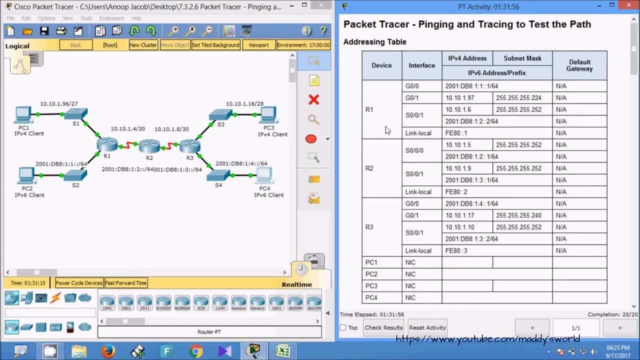 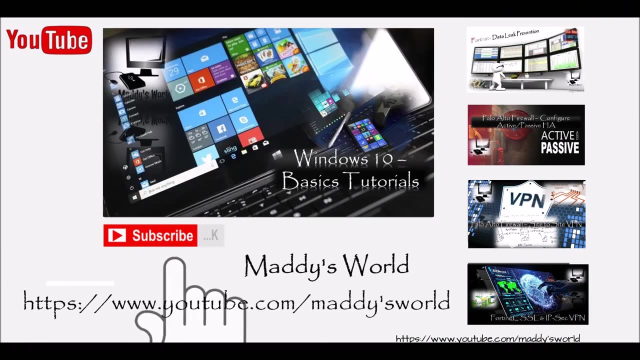 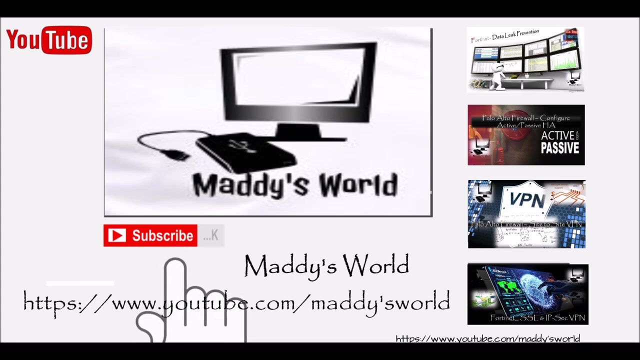 any doubt, please comment below. also, if you like my video, give a thumb and don't forget to subscribe the channel so that you will get latest uploading video info into your gmail. thank you, you you.